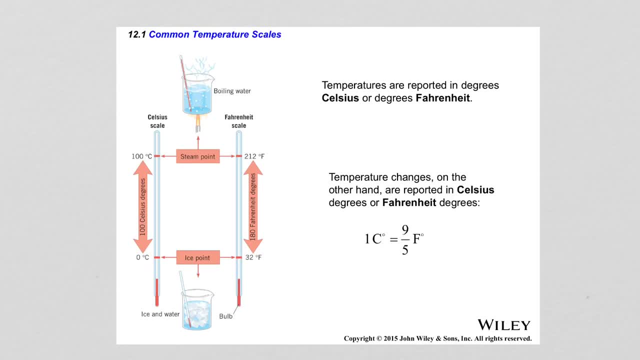 mixture, and, in labs, mercury instead of alcohol water mixture. Temperature is measured based on two temperature scales that are common in existence today: The Celsius scale, which is adopted by the metric system, and the Fahrenheit scale, which is adopted by the imperial system. Both measurement systems for temperature are based on two very specific 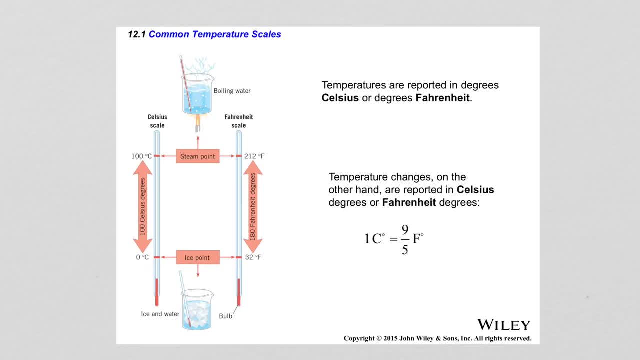 points related to properties of water. We have the freezing point of water, which for the metric system is zero degrees Celsius and for the Fahrenheit system is 32 degrees Fahrenheit, And the other point is the boiling point of water, which is 100 degrees for the Celsius system and 212 degrees for the 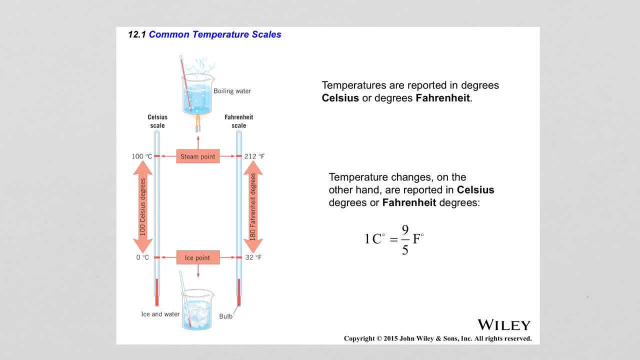 Fahrenheit system. So as you can see here, in the Celsius system there is exactly 100 degrees between the freezing and the boiling point, and for the Fahrenheit system there are 180 degrees between the freezing and the boiling point. So that means that that 1 Celsius degree is equal to 9 fifths of a Fahrenheit degree. 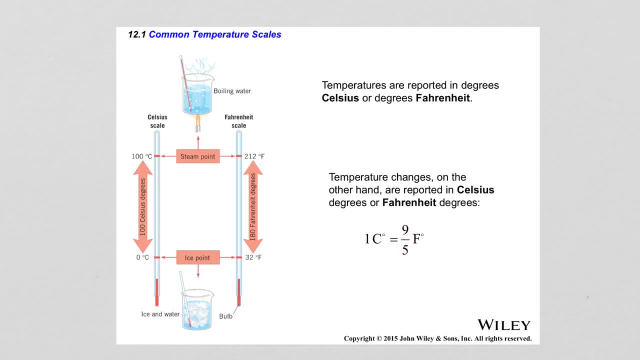 The correspondence is not one-to-one. So if one would want to convert between the two temperature scales, there are two convenient formulas that relate those two scales that can be used For conversion from Fahrenheit to Celsius degrees. take the temperature in Fahrenheit, subtract 32 from that. 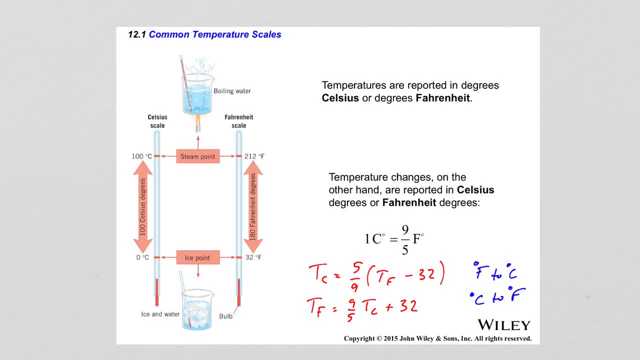 and then multiply by 5 and divide by 9.. For a conversion from Celsius to Fahrenheit, take the temperature in Celsius, multiply by 9, divide by 5, and then add 32 to that. So these are the two formulas that are used to convert between the two measurement systems for temperature. 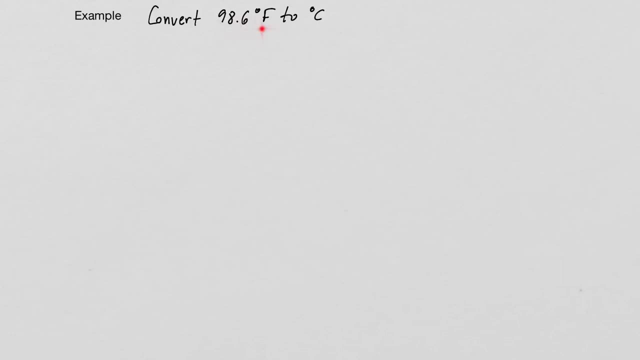 Let's do the following example. Let's convert 98.6 degrees Fahrenheit to degrees Celsius. The formula for conversion is that the temperature in Fahrenheit minus 32, multiplied by 5, divided by 9, will give me the temperature in Celsius degrees. 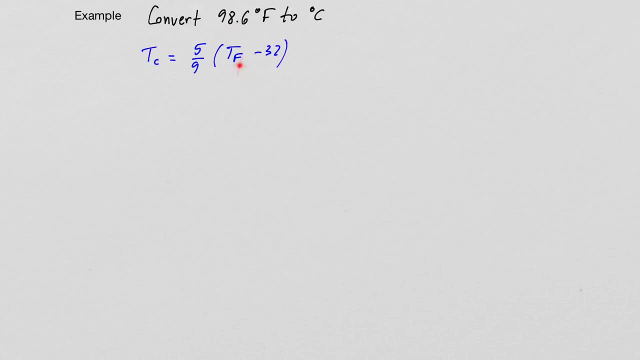 So let's substitute 98.6 degrees Fahrenheit in the formula and let's calculate the result. So I get 5 ninths times 98.6 minus 32, that is 5 ninths times 66.6, that gives me 37 degrees Celsius. 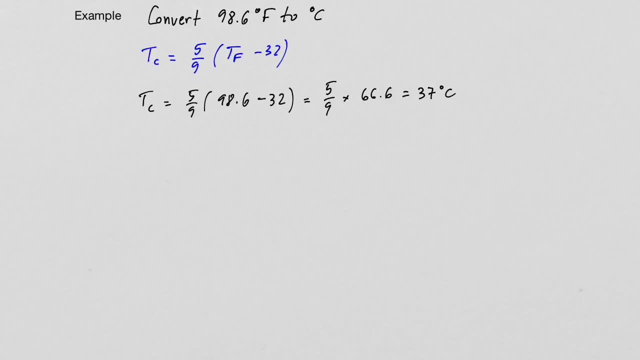 So in Celsius degrees, this is the temperature of the body, the body of an average human sized person. Let's do one more example. Let's convert negative 20 degrees Celsius to Fahrenheit. The conversion formula states that the temperature in Fahrenheit will be equal to 9 fifths the temperature in Celsius, plus 32.. 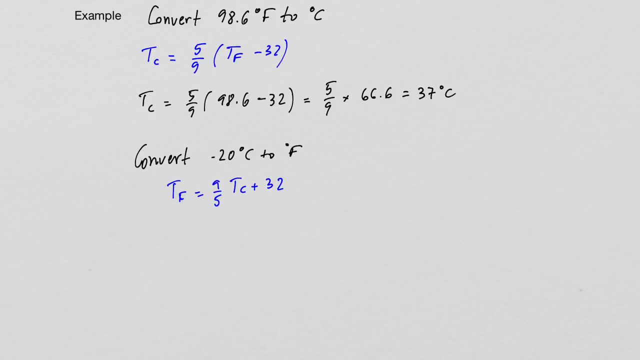 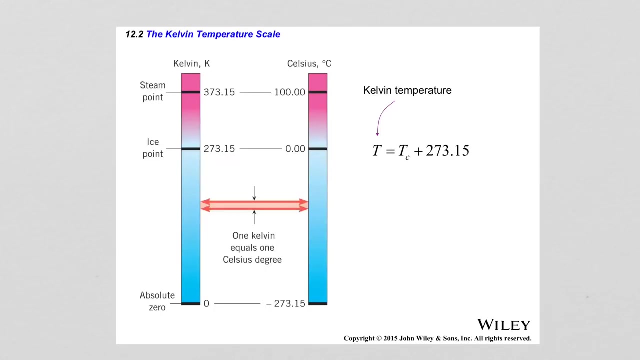 Let's substitute negative 20 in the formula and let's see what we get. So we get 9 fifths times minus 20 plus 32 gives me minus 36 plus 32, that is negative 4 degrees Fahrenheit. The Fahrenheit and the Celsius scales are very popular. 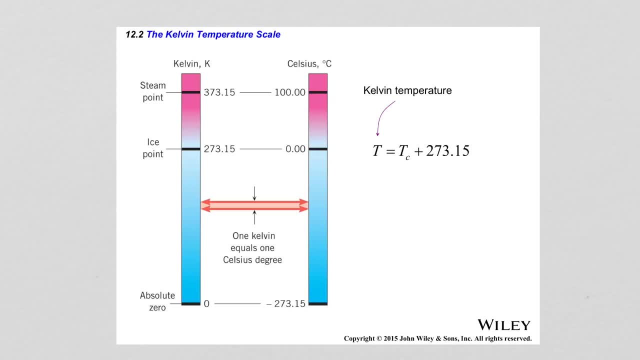 and very commonly used in everyday life, because the way that they are defined makes it very convenient to measure and describe typical ranges of temperatures that we are used to deal with. However, in many scientific applications and in situations where temperatures are very low or really high, 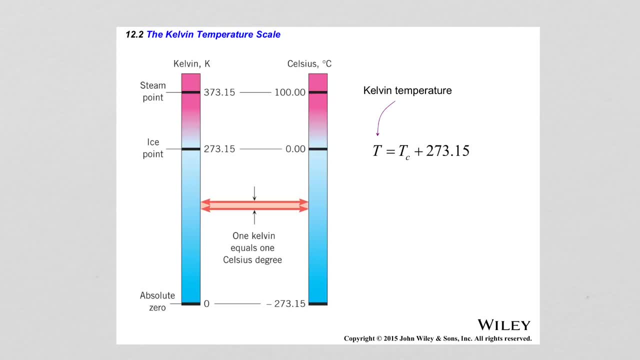 it is more convenient to use a different temperature scale, and that is the Kelvin temperature scale. The Kelvin temperature scale is also known as the absolute temperature scale, because it turns out that measuring the lowest possible temperature that can exist in nature is gives us a zero on the Kelvin temperature scale. 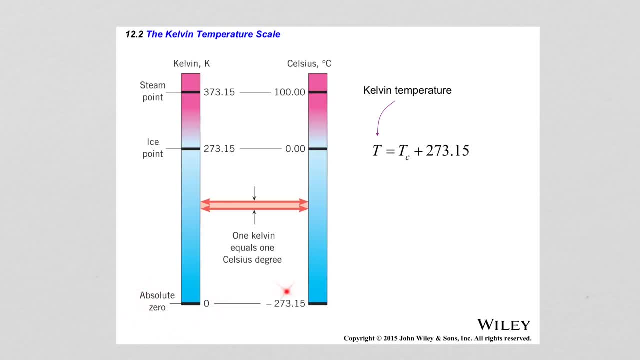 and that is how it's defined- which corresponds to negative 273.15 degrees Celsius. The name of this temperature scale, of course, was not randomly selected. It was introduced by the Scottish physicist William Thomson, also known as Lord Kelvin, So he was able to define this temperature scale. 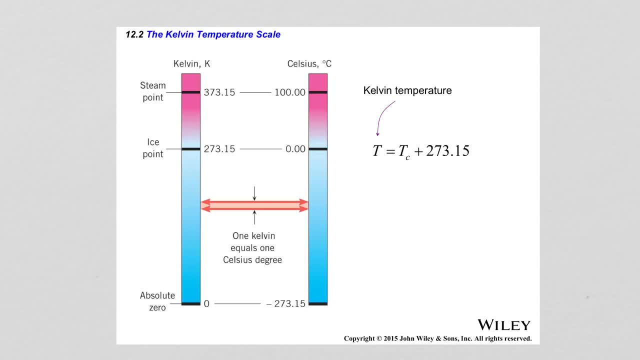 in terms of lowest possible temperature achievable, and thus his name is used for this scale. So again, the lowest possible temperature that can be achieved in nature, that can exist in nature, is the absolute zero. There is no lower than that, and that is the zero of the Kelvin temperature scale. 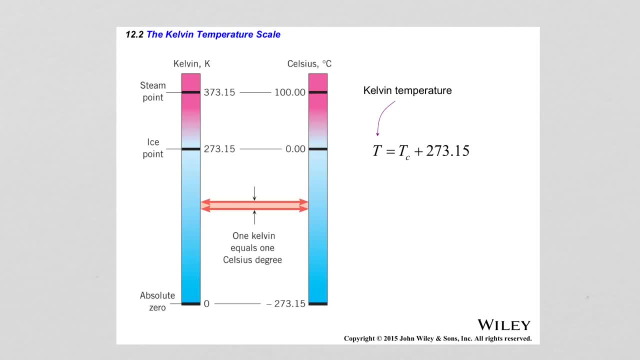 The Kelvin temperature scale is related to the Celsius scale and on the Celsius scale the absolute zero temperature corresponds to negative 273.15 degrees. The symbol for temperature in the Kelvin temperature scale is K and the relationship between temperatures in the Kelvin scale. 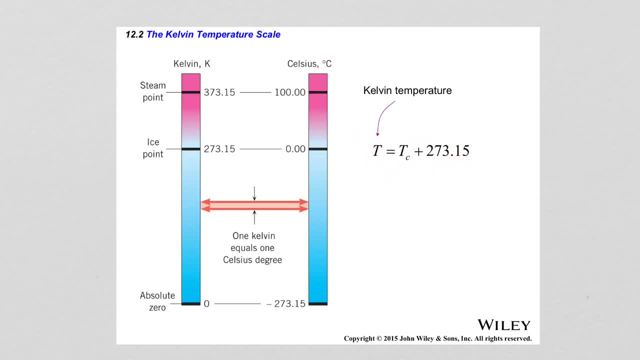 and the Celsius scale is given by this formula here. So the temperature in Kelvin is equal to the temperature in Celsius plus 273.15.. So the reason why we use Kelvin, apart from the Celsius scale, is that for the definition of certain thermodynamic properties, 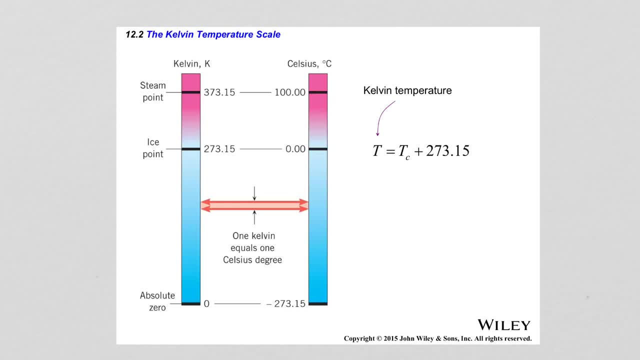 related to operations of engines and calculation of various physical quantities. the temperature in Celsius degrees does not give a proper result. The results are not accurate. However, if a switch is made using this conversion formula to Kelvin, the Kelvin temperature scale, then those physical quantities are defined properly. 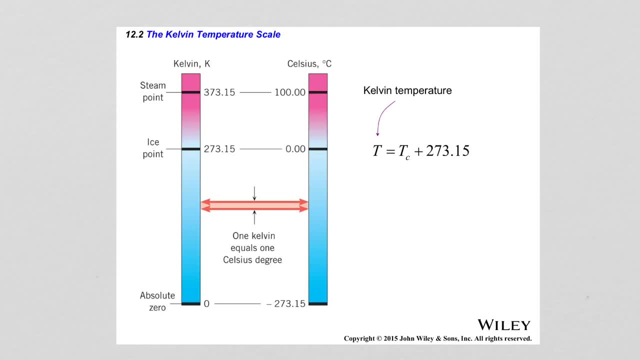 and calculations with those yield correct results. For example, in the chapter on thermodynamics, when I discuss heat engines, the concept of efficiency will require conversions of temperatures from Celsius to Kelvin in order to achieve correct results. Many materials have properties that are dependent. 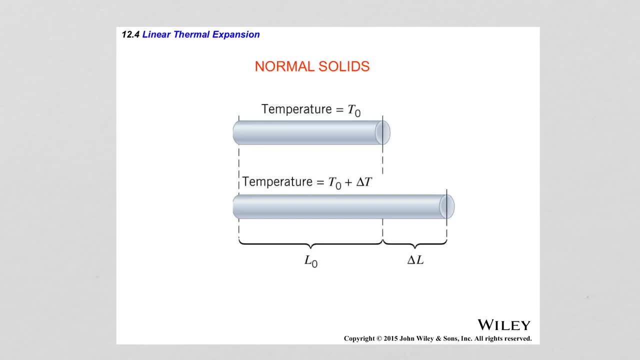 on the temperature of these materials. For example, for metals, with increase in temperature the resistance to conducting electricity increases. with decrease of temperature the resistance to conducting electricity decreases. So when metals are colder or cooler it's easier to conduct electricity through them. 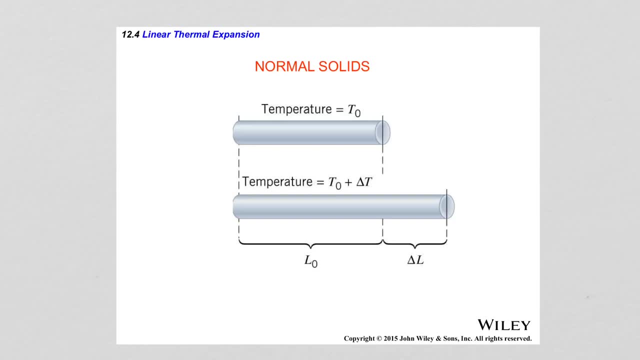 compared to when they are hotter For various rubbers and plastics. when they are at lower temperatures they are less elastic, less flexible and more brittle, and when they are at lower temperatures they are less flexible and more brittle as opposed to at higher temperatures. 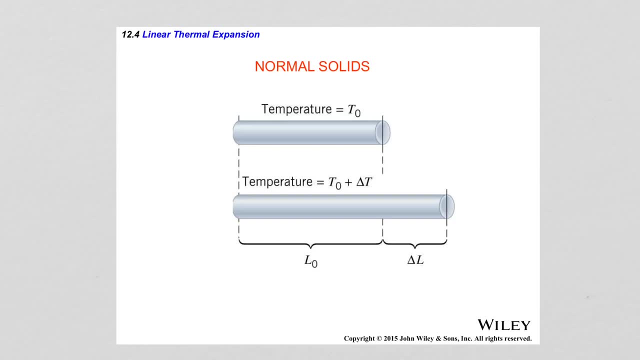 they are more pliable, more flexible, less brittle. One important property of solids is the linear thermal expansion. So for normal solids, if we have, let's say, a piece of metal bar at some initial temperature T0,, this metal bar will have some length- L0. 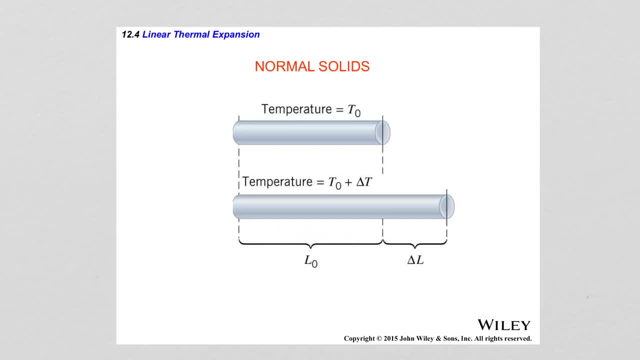 However, if the temperature of the bar is increased by the amount delta T, then the length of the bar will change by the amount delta L. Of course, if the temperature of the bar is decreased by delta T, then the length of the bar will decrease by the amount delta L. 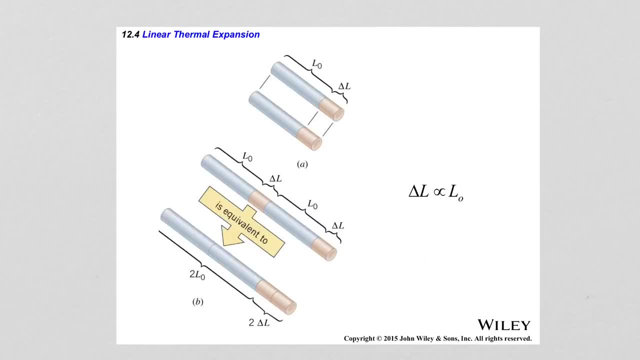 If I take two identical metal bars with starting length L0 and increase their temperatures by the same amount delta T, then their lengths will increase by the same amount delta L. Then if I had a bar that had double the length of each of the original bars, 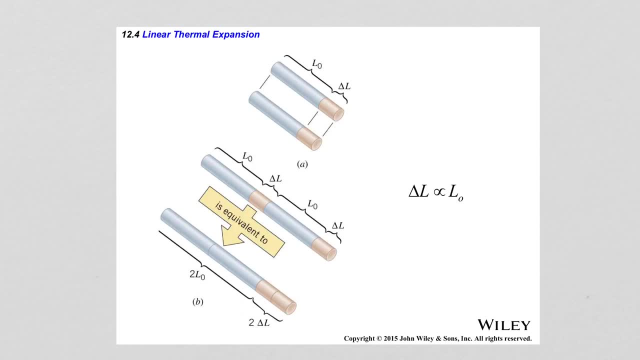 and I had it at that same initial temperature, T0, and increased the temperature by the same amount- delta T, then the change in length of that new bar would be double the change in length of each individual bar. So that means that I can define a formula. 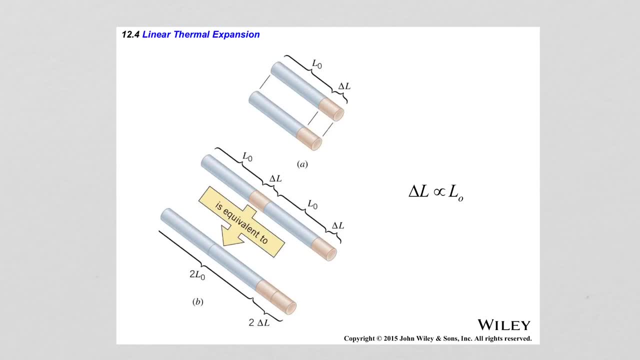 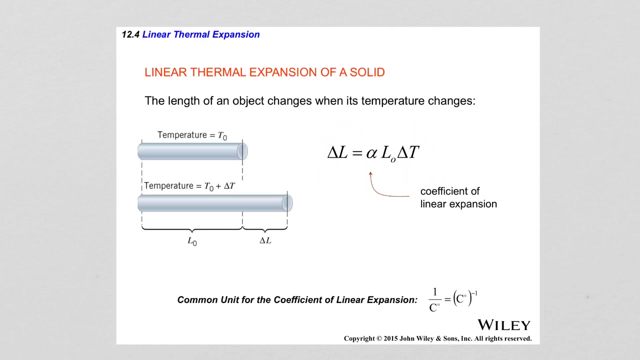 that is universal for linear thermal expansion of any solid and I can use it to calculate the relationship between: to calculate the change in length when a certain change in temperature occurs. So this relationship is given by this formula right here, The change in length is equal to. 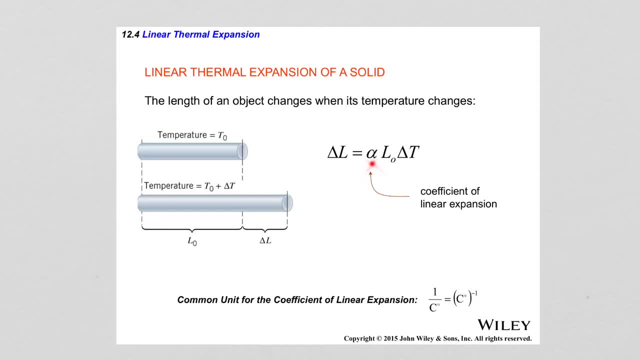 the product of the coefficient of linear expansion alpha, the initial length of the solid and multiplied by the change in temperature. The coefficient of linear expansion in the metric system commonly is measured in units of Celsius degrees to the negative first power. This formula here can be applied for any solid. 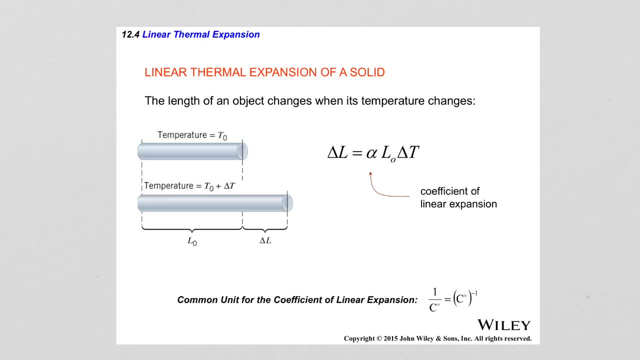 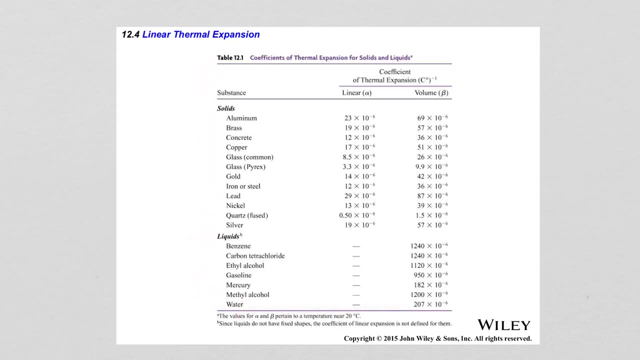 no matter what material it's made from. Coefficients of linear expansion are available in tables, For example in the textbook. the table for the coefficients of expansion are presented in this table. For solids, for various types we have the coefficient of linear expansion. 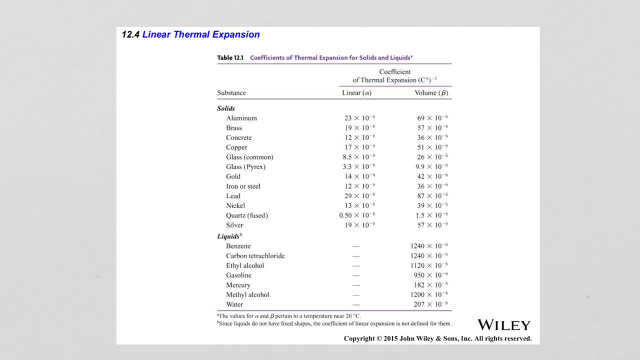 And of course for liquids. they do not expand linearly, they expand by volume only. So there's also values for the coefficient of volume expansion And I will discuss the relationship between change in volume and initial volume for any object when the temperature changes. 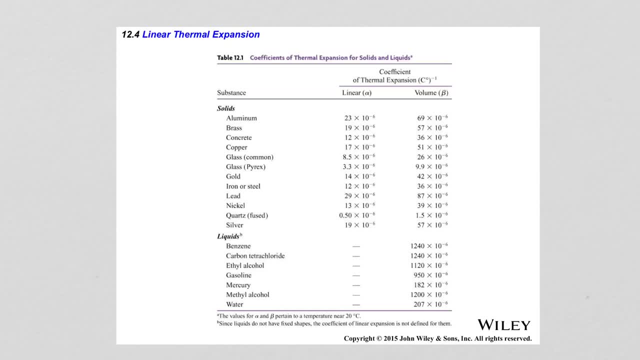 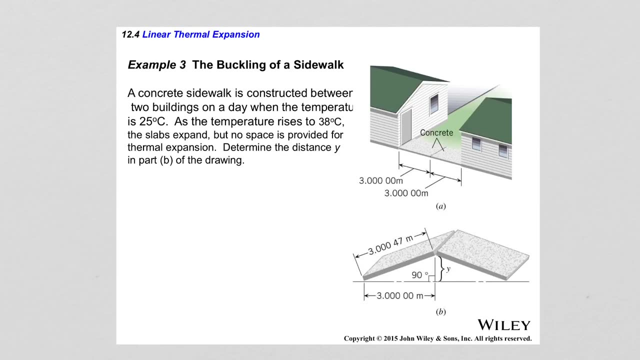 So let's look at the relationship between those things in the next few slides. First, let's look at one example of the application of the formula for linear expansion. A concrete sidewalk is constructed between two buildings. on a day when the temperature is 25 degrees Celsius. 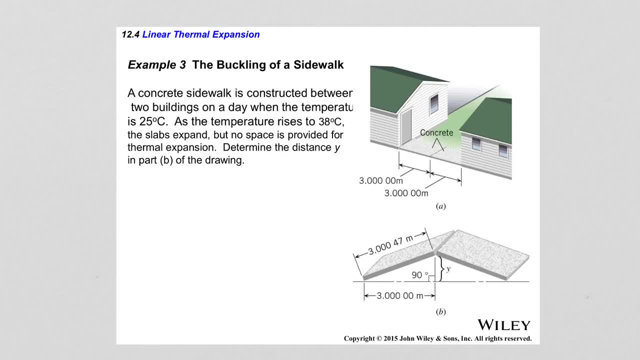 As the temperature rises to 38 degrees Celsius, the slabs expand, But no space is provided for thermal expansion. Determine the distance y in part b of the drawing. So here are the two concrete slabs with dimensions provided in the drawing. And so when the temperature is 25 degrees Celsius, 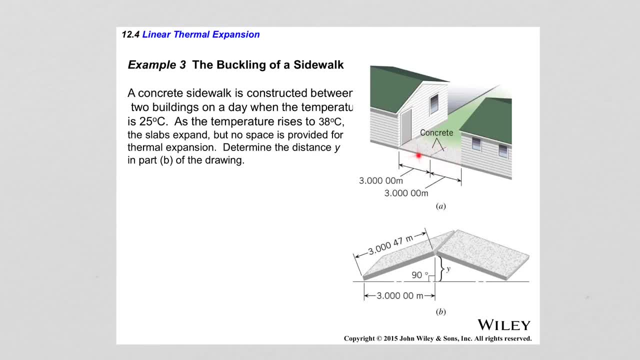 the two slabs are parallel to the ground. They're, you know, in contact with each other, But when the temperature reaches 38 degrees Celsius, due to expansion, the two slabs will angle, like so with respect to ground, And so each slab will be with length of 3.00047 meters. 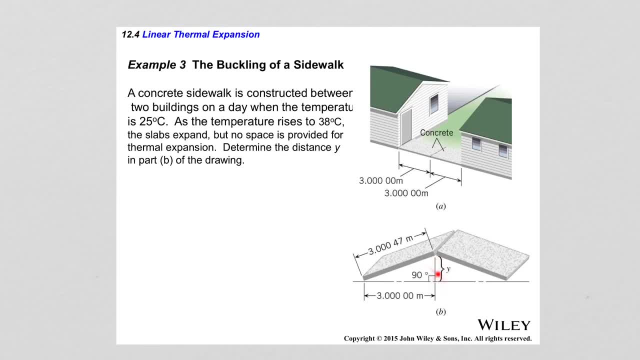 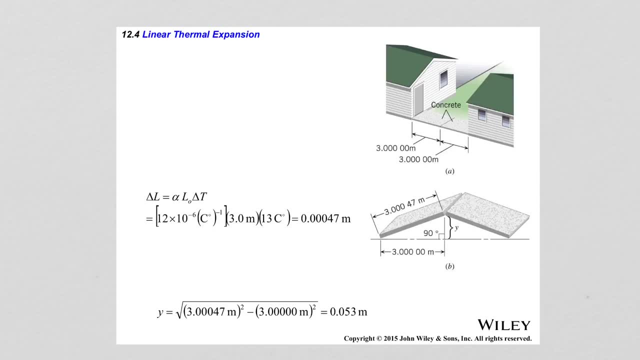 And the question is: what is this? length y above ground, So how it was determined that the length of the slab after expansion is 3.00047 meters. If I apply the formula for linear expansion, delta L is equal to the coefficient of linear expansion alpha. 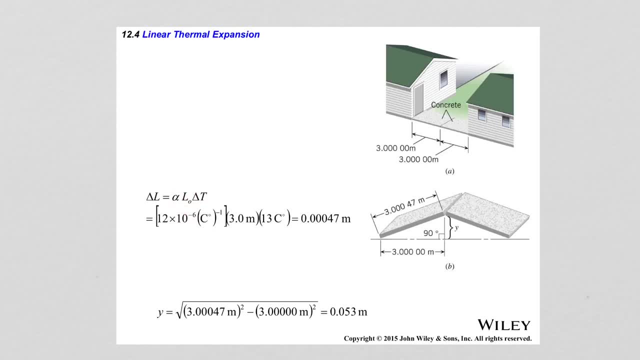 times the original length: L0, times the change in temperature to the slab. from the table for concrete, the coefficient of linear expansion is 12 times 10 to negative 6 Celsius degrees to negative first power times the original length of the slab: 3 meters. 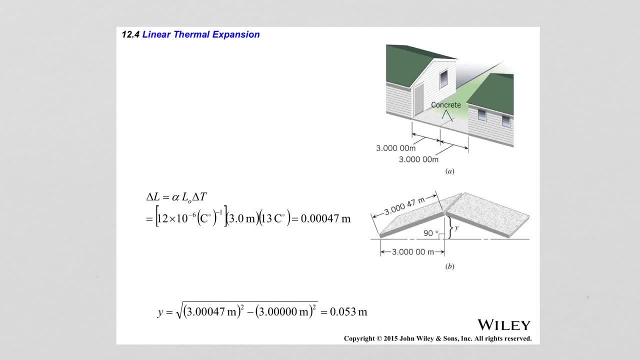 times the change in temperature, which is equal to 38 minus 25 degrees, so that is 13 Celsius degrees, gives me that the change in length will be 0.00047 meters. Now, from this drawing, here there is a right triangle. 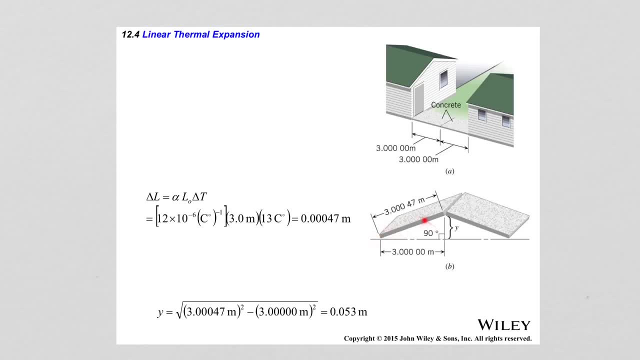 for which I know the base, which is 3 meters, and the hypotenuse, which is 3.00047 meters. So I can use the Pythagorean theorem to calculate the height of this triangle, which is the distance that is asked for in the question. 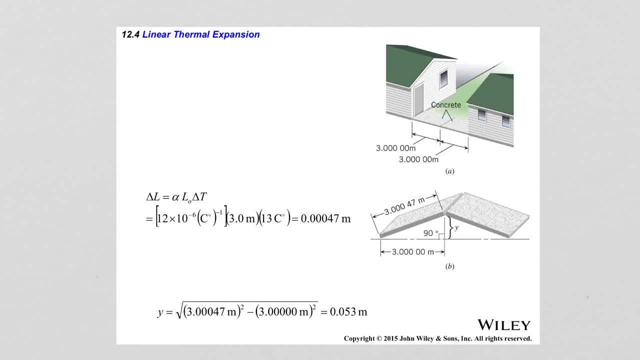 And this gives me 0.053 meters. This example is perfect to illustrate why, when you walk on a sidewalk, you see these grooves that are cut in the concrete every so often. These are meant for the effect of the linear expansion when temperatures change. 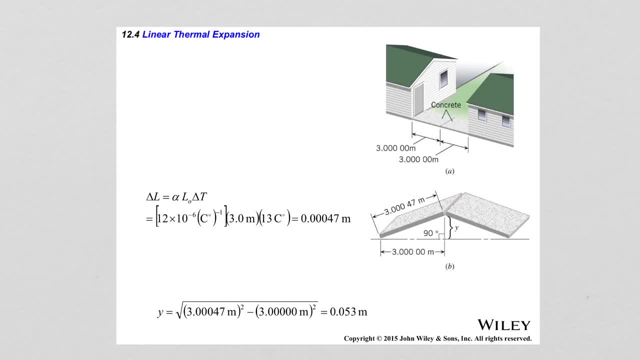 so that there is no damage to the concrete over time. Similar precautions are taken in building bridges. So there is this expansion groove, or joints that are built in the bridge. For railroad tracks, there is always a little bit of space left between sections of the track. 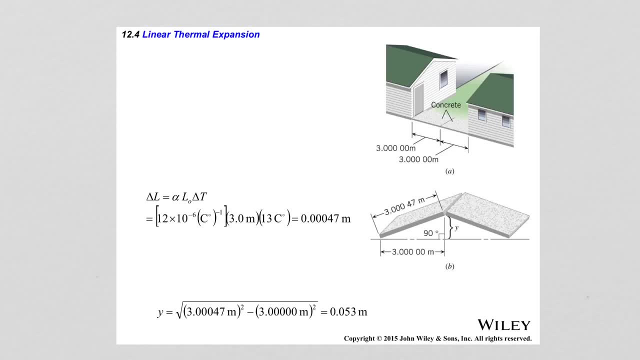 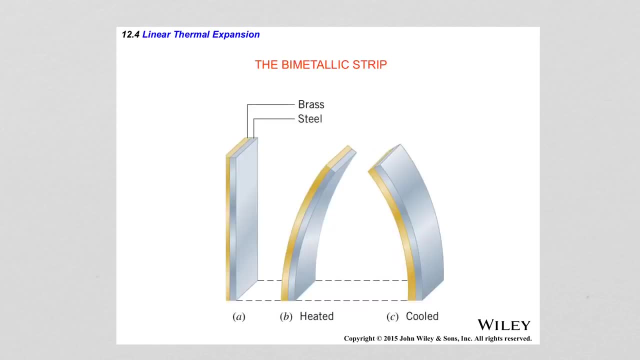 and so on and so forth. So all of these are meant to prevent damage during expansion when temperatures change. Here is another application of the properties of thermal expansion of materials. Many electronic devices have bimetal strips utilized in them. Bimetal strips are made of two different types of metal. 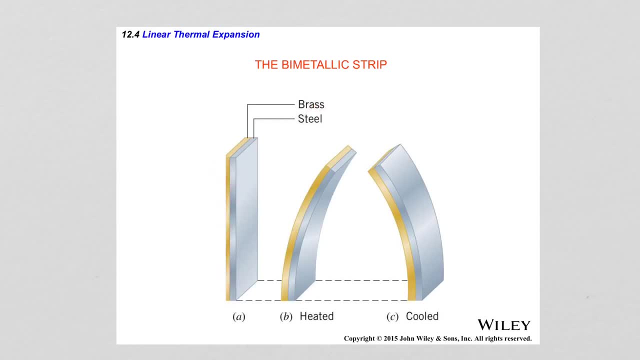 that are glued together, for example brass and steel, And, depending on the temperature, the two metals will expand or contract differently, which will cause the bimetal strip to bend one way or the other. This can be used for circuit breakers. 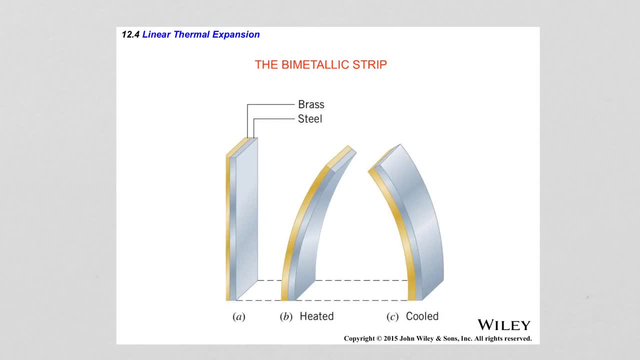 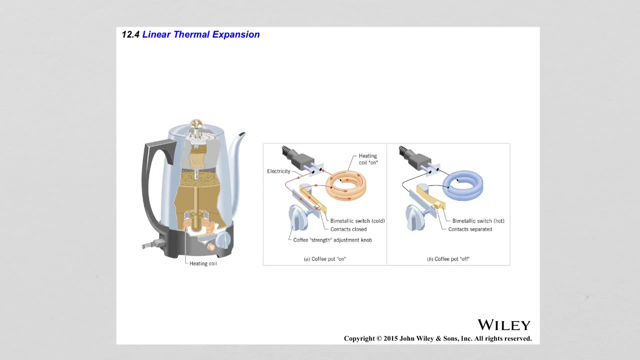 or switches for temperature controllers based on the programming of the particular device in use. So, for example, here we have an electric kettle where water is being heated and so electricity comes in through the power cord runs through the circuit here. the switch here connects to the bimetal strip. 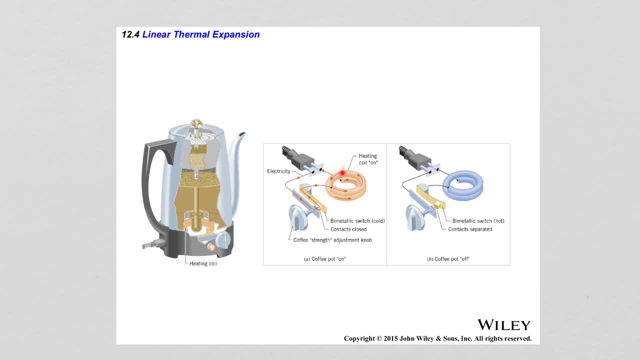 like so, and then the heating coil heats up the water inside. So once the temperature that is required is reached, this bimetal strip will start to expand, and because it's made of two different metals, they both expand at different rates. 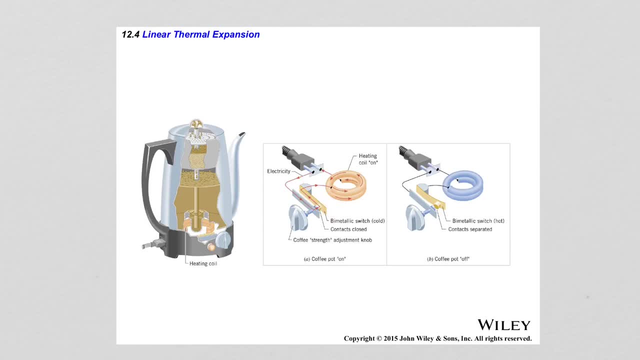 That will cause the bimetal strip to bend- In this case it bends away from the switch- and that disconnects the electric circuit. And so this is designed so that, when the water here is at its boiling point, this kettle will turn off automatically. 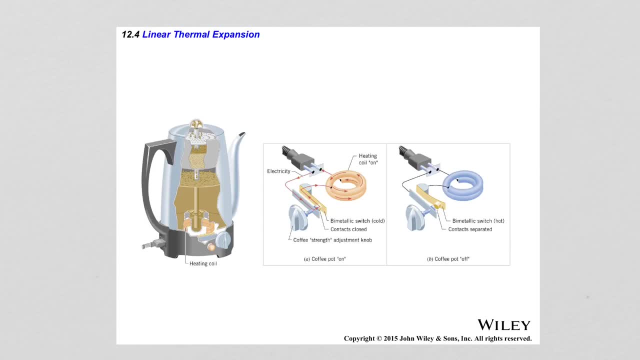 so that the water doesn't just boil off, And this, of course, is also a safety precaution against fires. Similar operation you have when you're dealing with your heating and cooling of your house. So the switch that turns on and off the AC. 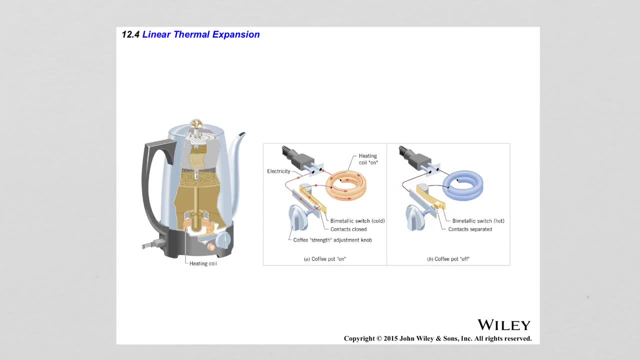 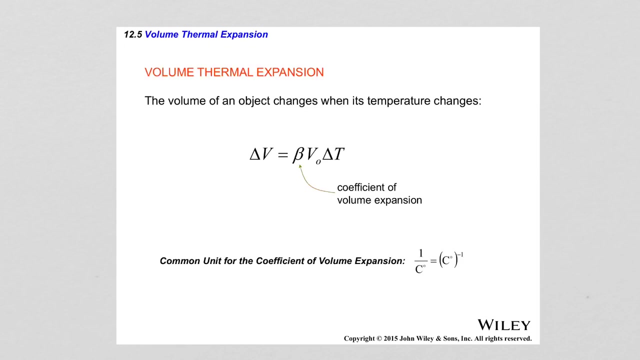 let's say, is essentially based on a bimetal strip design. Circuit breakers are also based on bimetal strip design, and there is also many other applications that have similar design, So solids can expand in one dimension. Of course, this is a good approximation. 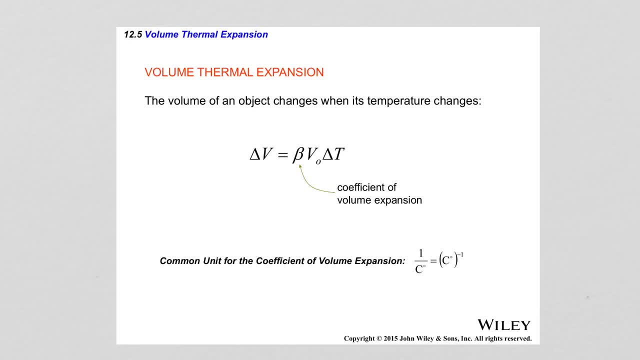 for a solid piece that is considered to be dimensionless and only has length, but it doesn't have a width or a height. However, in general, solids are three-dimensional objects, and so they, when heated or cooled, expand or contract in all three dimensions simultaneously. 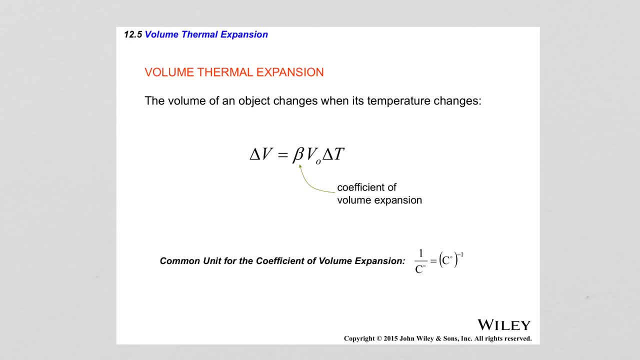 at the same time. So their volume changes when the temperature of a solid changes. When I discussed linear thermal expansion, I only discussed solids, and that is because liquids do not expand only linearly, They expand by volume, and for gases expansion is not even measured like that. 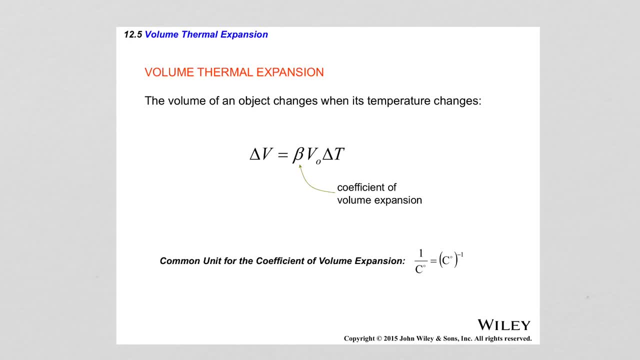 because the gas would take the volume of its container and so you can have the same amount of gas in different volume containers and therefore the volume of the gas would be different. So for gases we don't even talk about volume expansion, because their properties are not related to that concept. 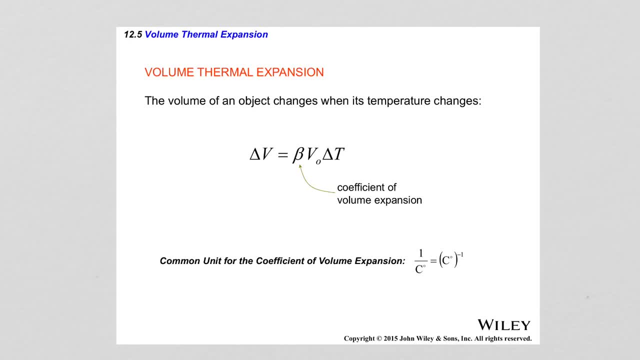 So volume expansion when change of temperature occurs is a property that solids and liquids experience, And the relationship between the change in volume and the original volume and the change in temperature is given by this formula here. So the change in volume is equal to the product of the coefficient of volume expansion beta. 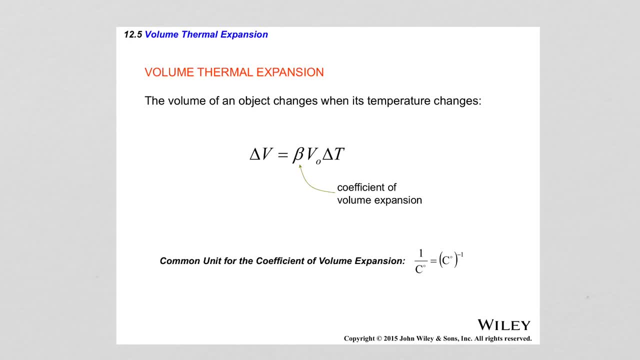 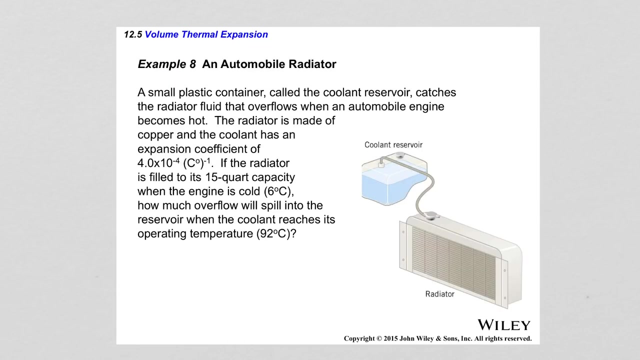 the original volume V0, and the change in temperature, T, A common unit or a more- a unit that's used more often than others- is for: the coefficient of volume expansion is degrees Celsius degrees to the negative first power. Here's an example that illustrates the application. 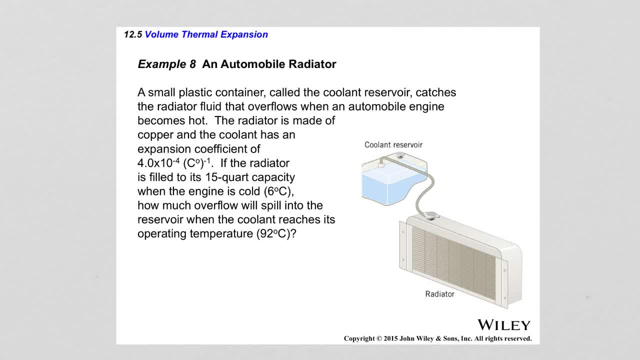 of the formula for volume thermal expansion. A small plastic container called the coolant reservoir catches the radiator fluid that overflows when an automobile engine becomes hot. The radiator is made of copper and the coolant has an expansion coefficient of four times 10 to the negative fourth Celsius degrees. 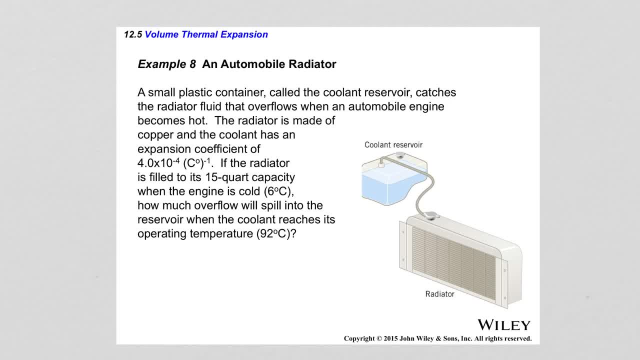 to the negative first power. If the radiator is filled to its 15 quart capacity when the engine is cold at six degrees Celsius, how much overflow will spill into the reservoir When the coolant reaches its operating temperature of 92 degrees Celsius? So to answer this question, 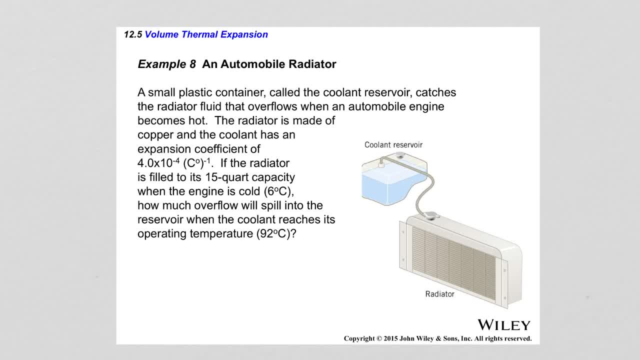 I need to calculate the change in volume for the coolant and the change in volume of the reservoir- I'm sorry of the radiator- And then take the difference and that's going to give me the amount of coolant that will overflow in the coolant reservoir. 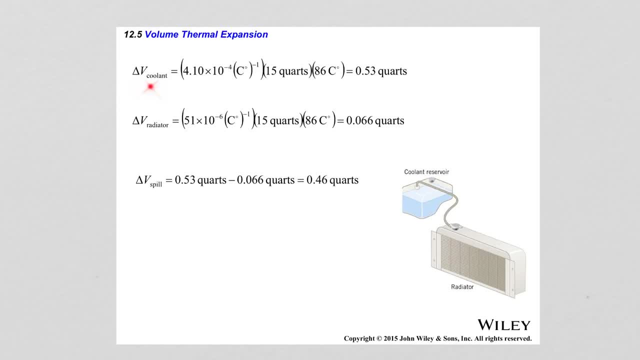 So for the coolant the change in volume is equal to the coefficient of volume expansion, which is four times 4.1 times 10. to the negative four Celsius degrees, to the negative first power times the volume of the coolant, 15 quarts. 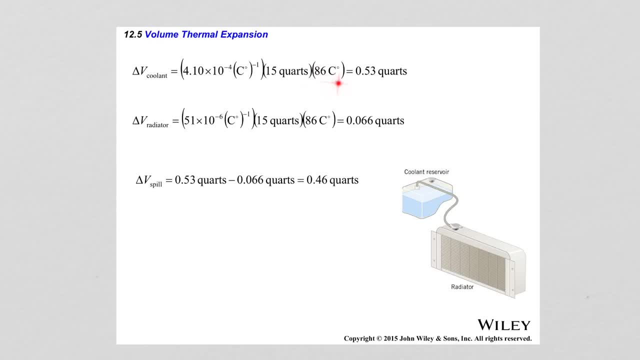 times the change in temperature, which is 86 Celsius degrees, and that gives me 0.53 quarts. So that's how much the volume of the coolant will change when the temperature increases from six degrees Celsius to 92 degrees Celsius At the same time. 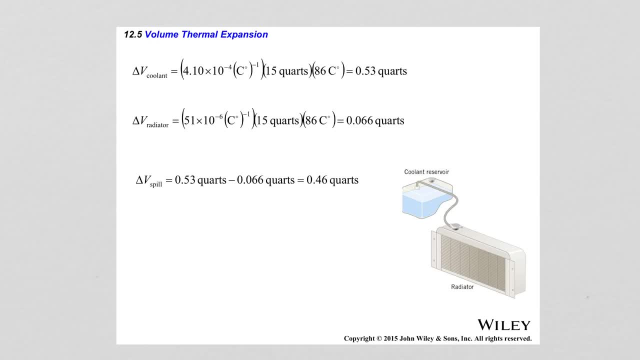 the volume of the radiator changes by 0.066 quarts. So that is the coefficient of volume expansion of copper 51 times 10. to the negative six Celsius degrees, to the negative first power times, 15 quarts times 86 Celsius degrees. 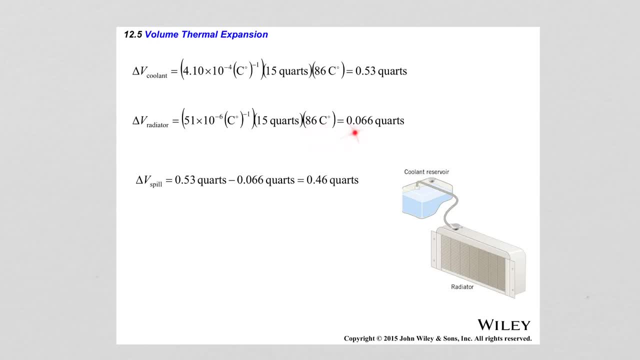 which is the change in temperature. So that is 0.066 quarts. So then the volume of coolant that is going to spill into the coolant reservoir is 0.53 quarts minus 0.066 quarts, and this is 0.46 quarts. 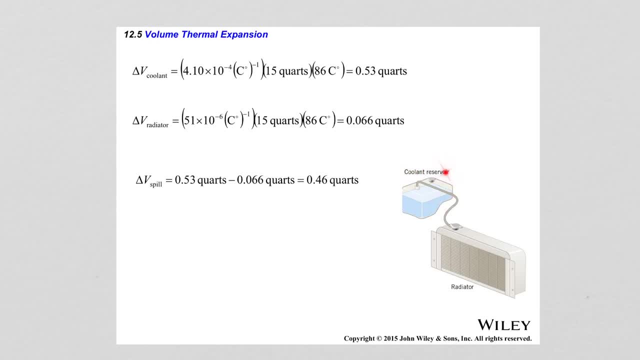 So all cars are equipped with a coolant reservoir where the antifreeze overflows due to the difference in volume between the antifreeze, the coolant and the radiator of your vehicle, And you can tell that the coolant will expand more than the radiator. 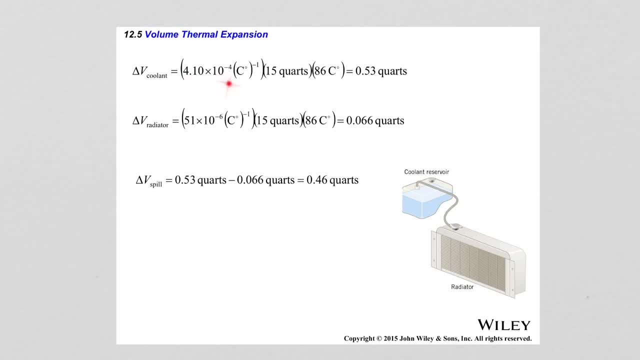 by just looking at the coefficients of volume expansion. As you can see, the coefficient of volume expansion of the coolant is of the order of 10 to the negative fourth, and the coefficient of volume expansion of the radiator is at the order of 10 to the negative sixth. 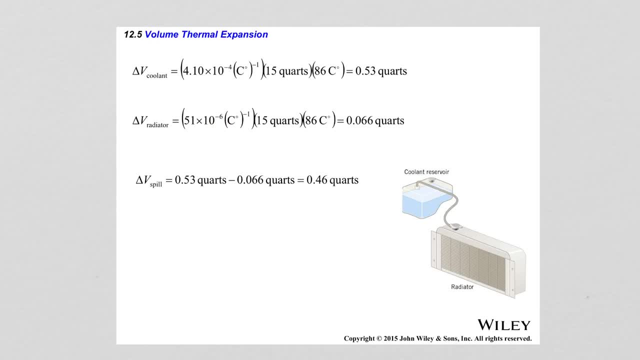 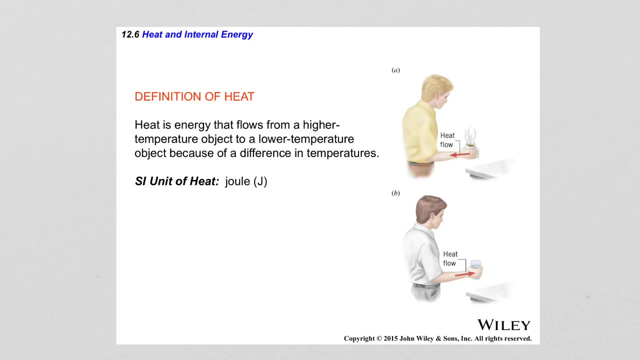 So the coolant roughly expands 100 times more than the radiator itself. Let's talk about heat and internal energy. now, For example, take an object that is hot, Let's say boiling water, that is placed in a glass and the temperature of boiling water is 100 degrees Celsius. 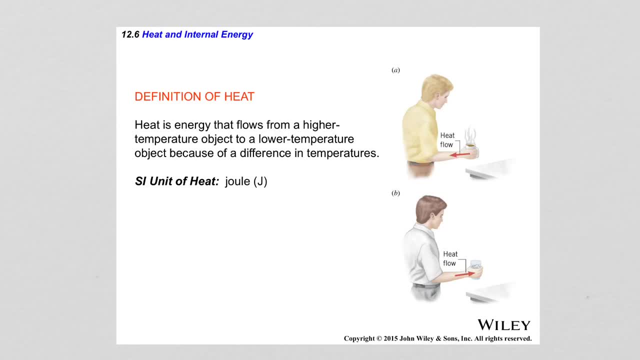 So we know that the temperature is high and we know that this water is hot. Well, after some time you would observe that the temperature of the hot water is going to be lower, so it decreases. Eventually it will reach room temperature. 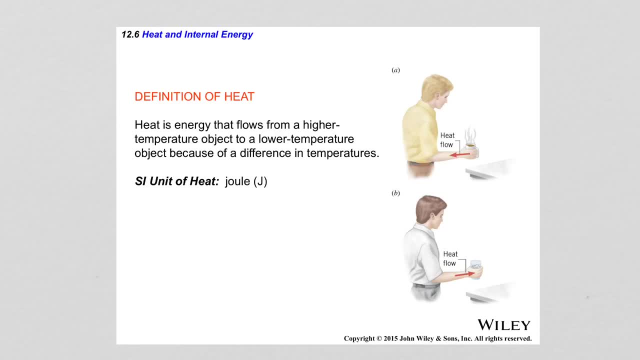 and then we say that the water is no longer hot. Let's say we can call it cool. Now, if you place this glass with water in the fridge, the temperature will go down even more, and now the water will be what we call cold water. 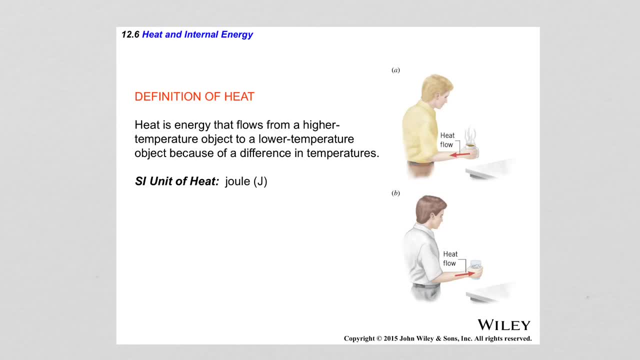 So the temperature of an object determines whether the object is hot or cold, according to our understanding of what that means. But how did this object became cold when it was hot? The reason for that transition was because heat left the object and was dissipated into the environment around it. 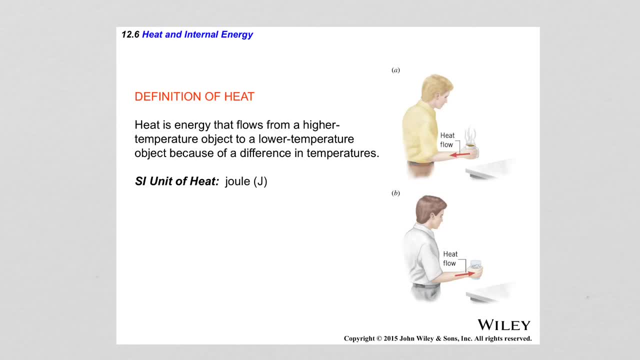 Heat is defined as the energy that flows from a higher temperature object to a lower temperature object because of difference in temperatures, And this can be demonstrated by taking two identical objects, for example, two identical cubes made of steel, one, let's say, at 100 degrees temperature. 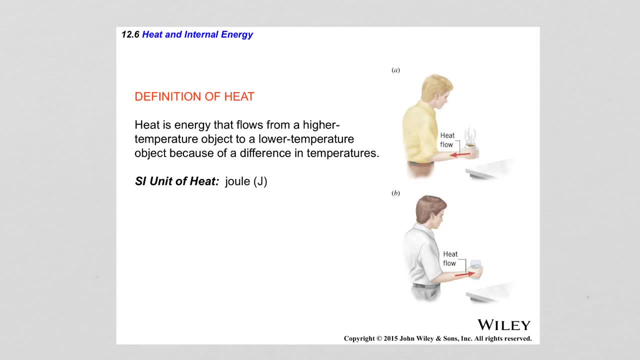 the other one at room temperature. When those two blocks or cubes are placed in thermal contact, meaning they are physically in contact with each other, you would observe that the hotter cube is going to cool down, while the cooler cube is going to warm up. 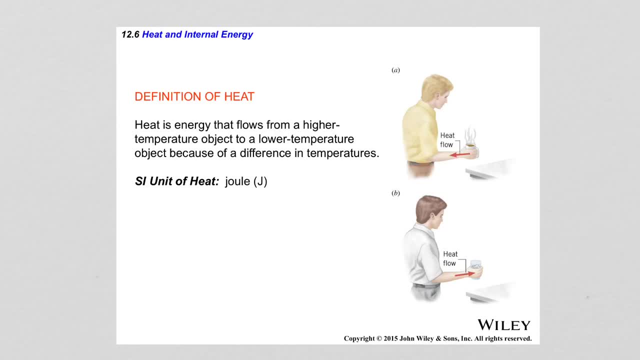 Eventually both will have the same temperature. So that means that heat leaves the hot cube and enters the cool cube. So heat flows from the hotter object to the colder object, And of course you can conduct an experiment in which you have a cold object and a hot object. 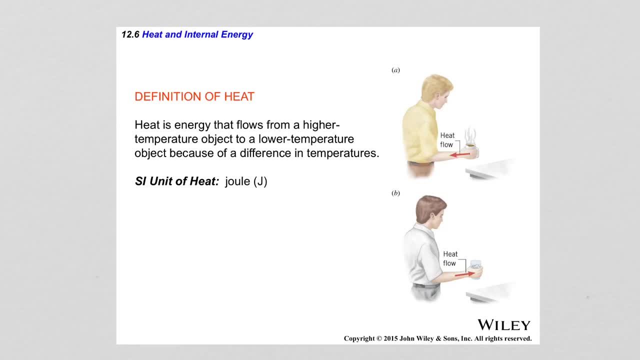 bring them in contact and you will see that you will never achieve a result in which the colder object becomes colder and the hot object becomes hotter due to heat flow from the cold object towards the hot object. So the direction of heat flow is always. 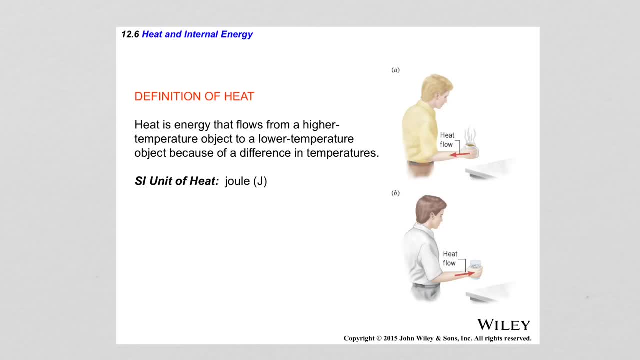 from the hot object to the cold object. That is the natural direction of flow of heat energy. The heat that flows from hot to cold originates in the internal energy of the hot substance. So what is the internal energy of the hot substance exactly? For a solid, that would be the energy with which the molecules 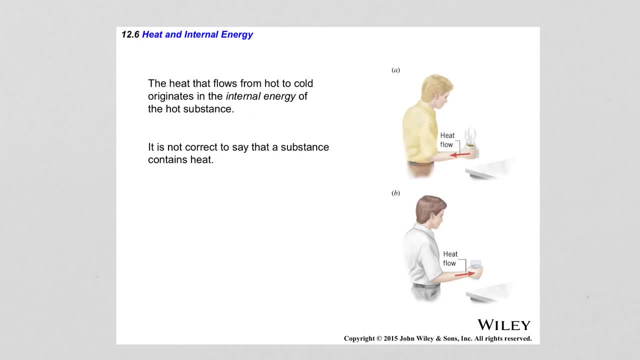 or the atoms from which the solid is made, are oscillating about their equilibrium positions. So the hotter the object, the higher the energy of oscillations, the higher the internal energy of that object. For gases, the internal energy is contained in the kinetic energy. 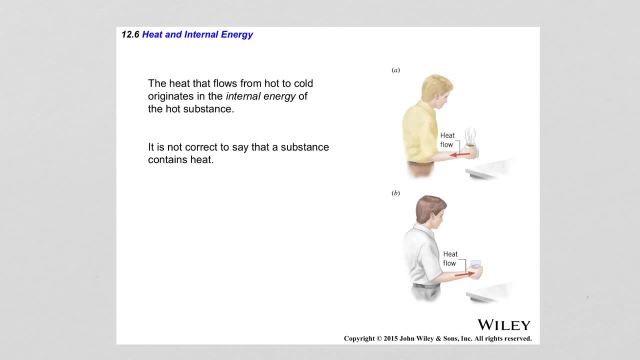 of motion of the molecules of the gas, the potential energies of interaction between the individual molecules, rotational kinetic energies of the molecules and vibrational energies of the molecules. So for gases the internal energy is a more complex quantity compared to solids. However, for either type of substance, 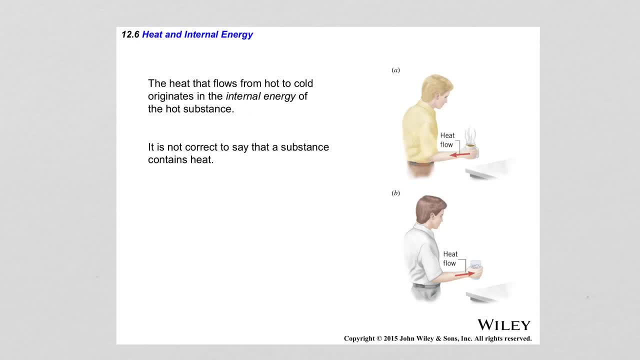 the internal energy is associated with some energy property of the molecules or atoms or the building blocks of those substances. So in this sense it is incorrect to say that heat is stored in a substance. What is stored, if you will, is the internal energy of the substance. 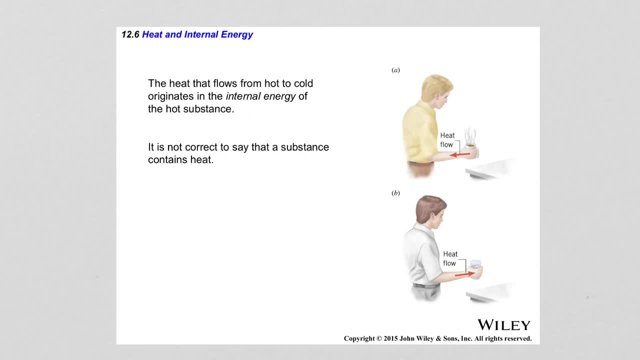 And so then, how is the heat transferred from an object with higher internal energy, or hotter object, towards an object with lower internal energy or colder object? For solids, that happens through mechanical collisions between the atoms or molecules of the hotter solid and the colder solid. 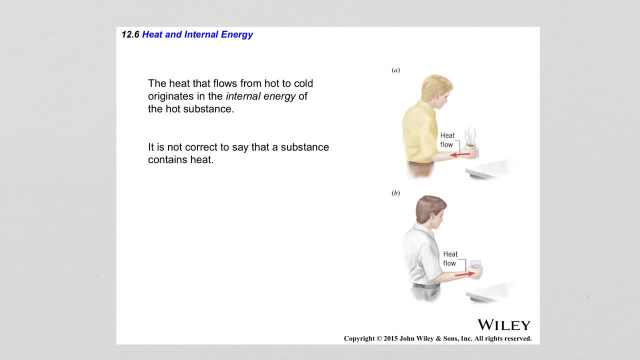 So through those collisions the internal energy of the hotter object is being transferred towards the internal energy of the colder object until both energies are the same. At this point transfer doesn't occur anymore. For fluids, the transfer of energy happens through introducing heat in the system. 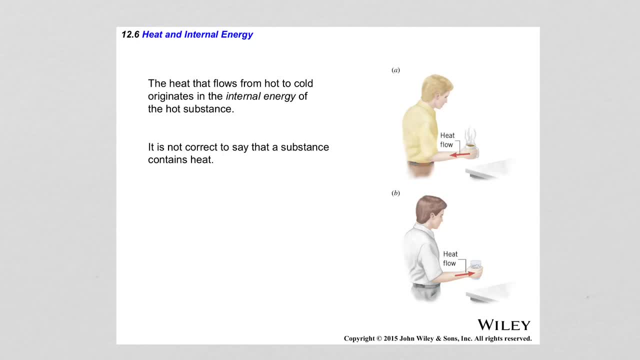 and causing the molecules that are closer to the heat source to move faster and faster and faster. That makes them move away from the heat source And then, in the empty space closer to the heat source, molecules that were initially further away will come closer due to just a random nature of motion. 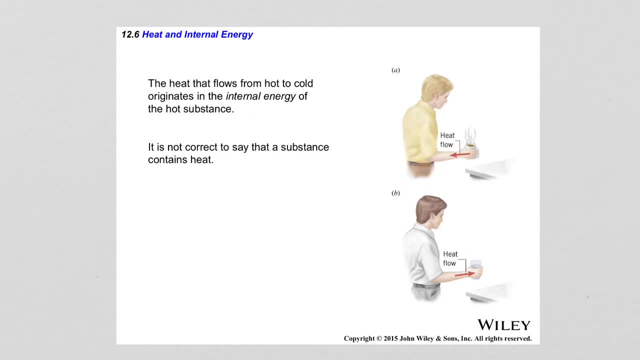 They will receive more kinetic energy, more rotational energy, more vibrational energy. They will move away. Others will come in, They will receive more energy, move away, And so you can think of the way that heat is transferred inside a liquid or gas. 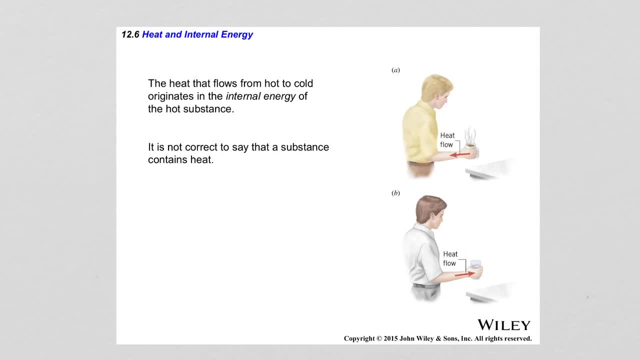 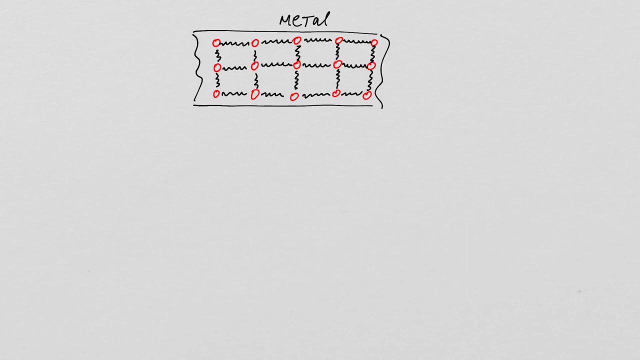 as a current that sort of circulates inside this fluid, And so this is known as convection current. So let's illustrate these concepts of heat transfer for solids and for fluids with two simple drawings. So here's a piece of metal. You can think about it as a metal bar. 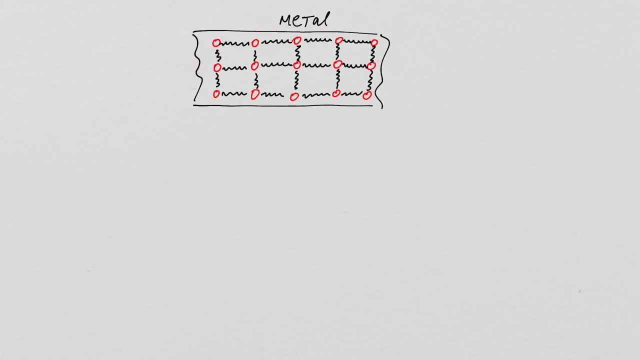 or a metal wire, It doesn't matter Which has a periodic lattice structure where the atoms are arranged in nice, neat symmetric arrangements like so, And the forces that these atoms interact with are represented with those tiny springs. So at all times these atoms pull and tug on each other. 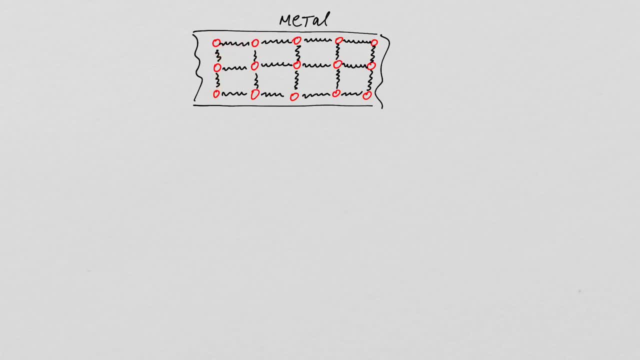 through those springs, either stretching a little bit or compressing a little bit. So if I introduce a heat source here, let's say bottom left corner, what that is going to do is going to start to increase the temperature of this lower left corner. 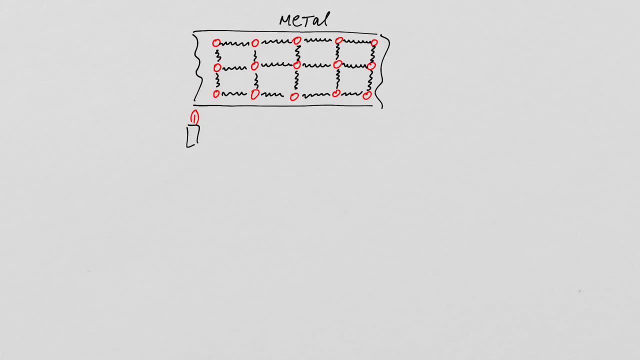 Well, how does this atom feel this increase in temperature? Well, this atom is going to vibrate more vigorously, with more deflection from its equilibrium position, And that of course happens in all directions. It's a three-dimensional vibration. But then, through those connections with these forces here, 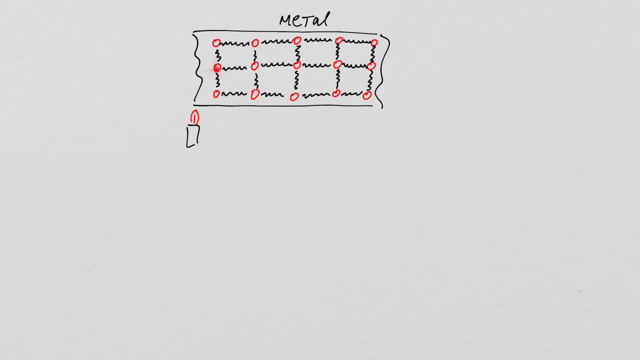 with the neighboring atoms. these neighboring atoms will start to also oscillate more vigorously, with higher deflections, about their equilibrium positions, But then these are connected to their neighboring atoms, so they will also start to oscillate about their equilibrium positions more vigorously, But then they are connected to other atoms. 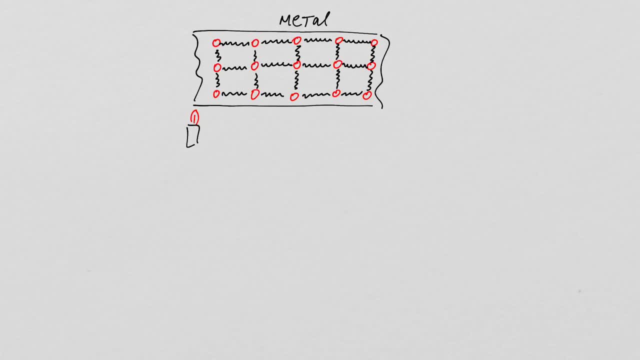 so those will also start to vibrate more vigorously, And so at some point the entire lattice structure will be oscillating at higher deflections from the, with high amplitude essentially, And we measure this effect as increase in the temperature of the entire metal object. 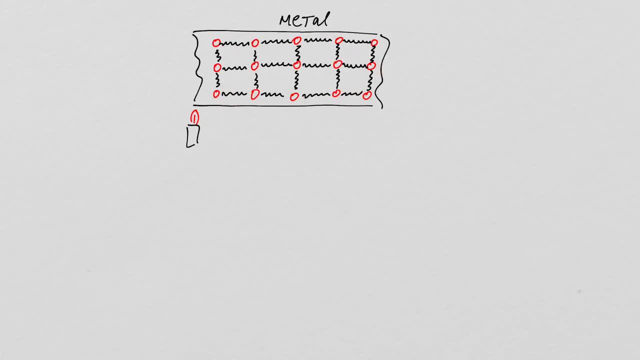 So now, if I placed another metal object in contact with this one right here, what's going to happen is these atoms that are in contact with the atoms of the other object, they will mechanically collide with each other, And so, when these collisions happen, 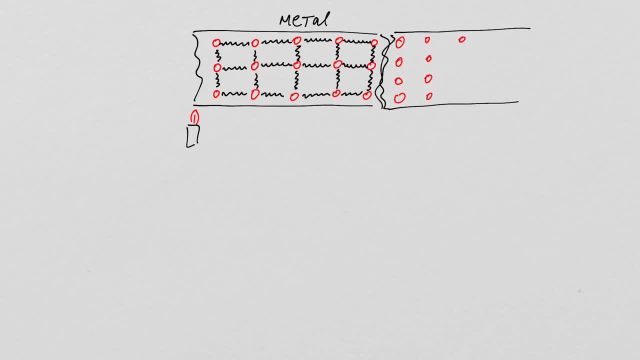 these atoms of the second piece of metal will start to also oscillate with larger amplitudes, And so then that is measured as increase in temperature of the second metal object. If I removed this heat source after some time, what happens is both of these. 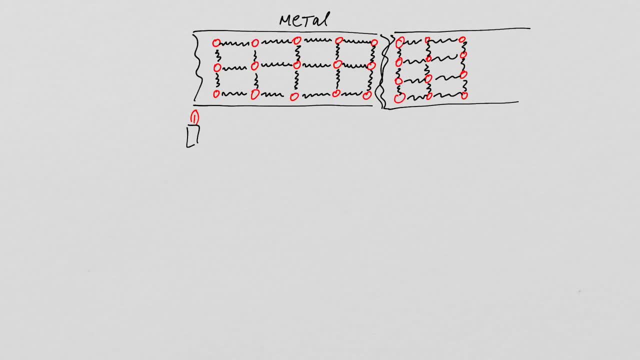 assuming that they initially are at the same temperature after the heat was introduced, both will start to lose energy. How is this energy lost? Well, around these metal pieces there is air, So the air molecules that are closest to the metal pieces will collide with the metal. 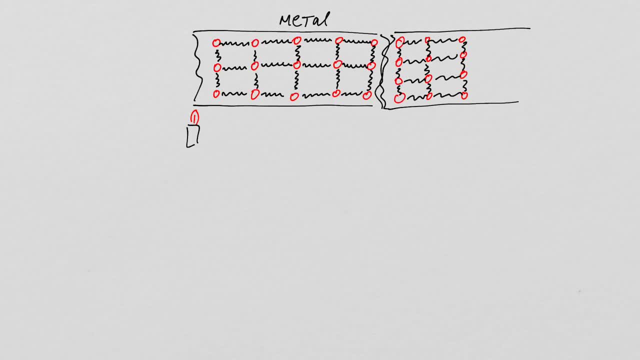 And then they will receive an energy boost, if you will, from the heat or the internal energy contained in these metal pieces. And so as the air molecules gain energy, the metal pieces lose energy. So, after enough collisions happened between the air molecules and the metal pieces, 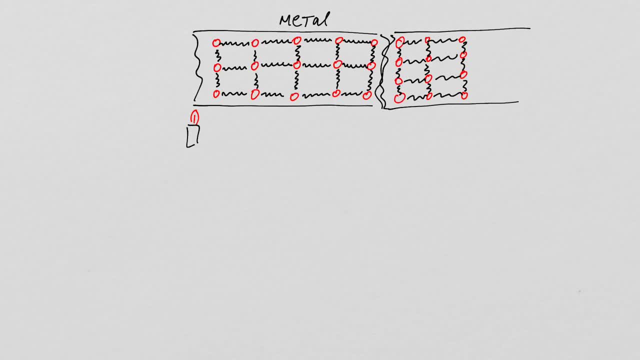 the metal pieces have lost enough energy for their temperature to be measured as lower temperature than before. And then eventually, after long enough time, the temperature of the air around the metal pieces and the metal pieces will be the same, at which point no longer they will be exchanging heat. 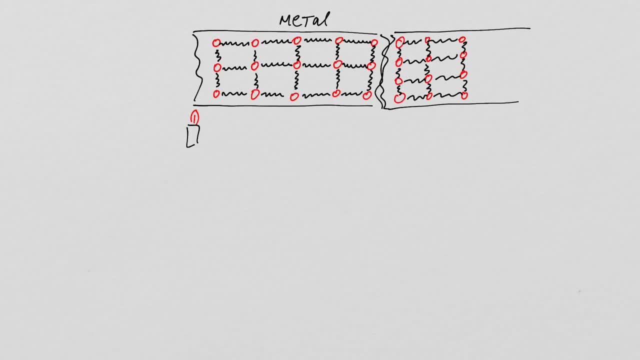 between the two substances, air, and the metal from which these wires were made. Now let's look at how gases and, of course, liquids are exchanging heat within themselves. So this is a container here that is closed, And let's fill it with some gas. 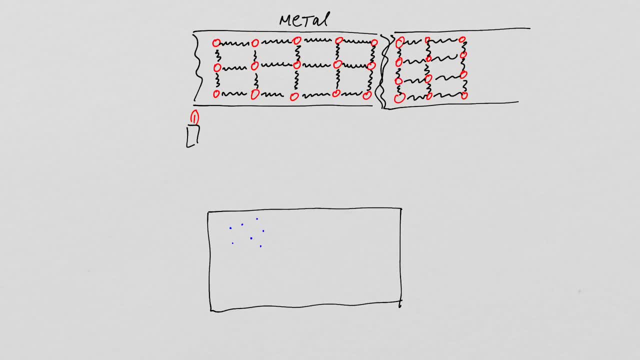 So we have gas molecules that are randomly moving inside the volume of this container. There is no preferred region here where the molecules will be more concentrated, So we can assume that initially, at room temperature, the gas is uniformly distributed inside the volume. So then I'm going to introduce a heat source. 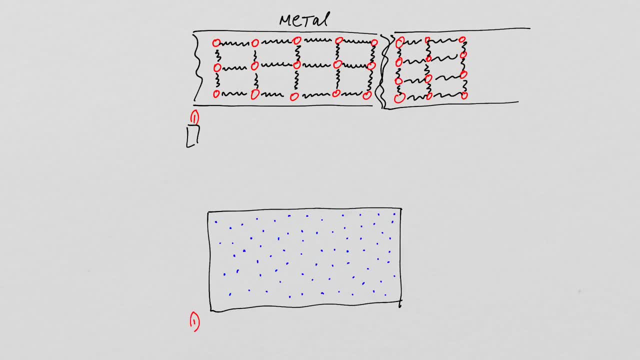 here at the lower left corner, which will result in heating up of the walls of the container right here in this region. So when these gas molecules collide with these walls, they will receive more energy and then they will in general move away from this area where. 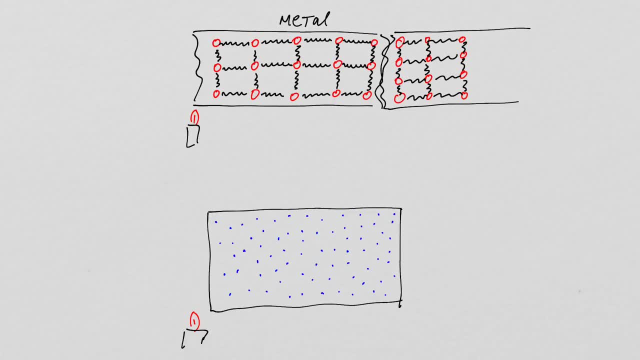 the walls are hotter. So some molecules will move in this general direction when they get more energy from interaction with the walls of the container. But then that leaves more room here that's empty. So of course molecules will move into in here and they will receive some energy. 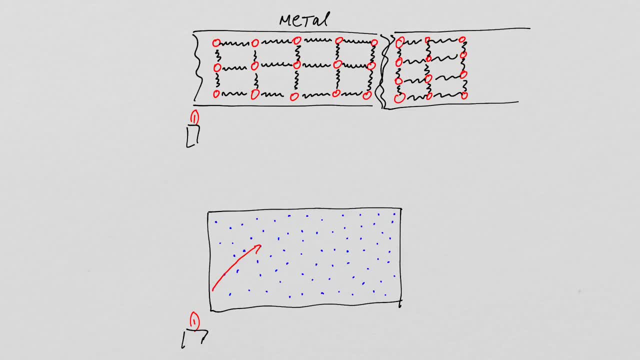 from the walls. So here we go. So molecules will come in here like that At the same time, the molecules that were initially energized. they will kind of move this way. They will collide with the walls of the container. They will lose some energy. 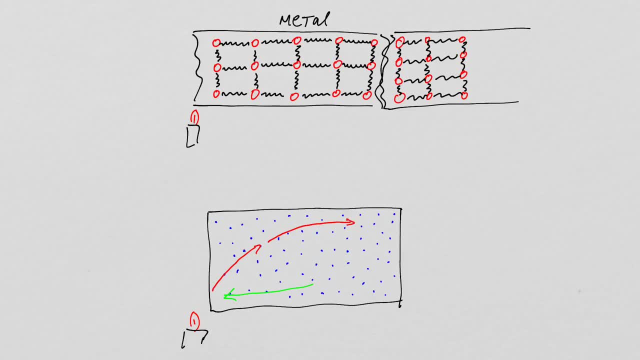 and then they will move randomly around, But at some point more molecules, but not at some point. but more molecules are coming in this way due to collisions with the hot walls, And therefore more molecules are coming the other way to take their place. 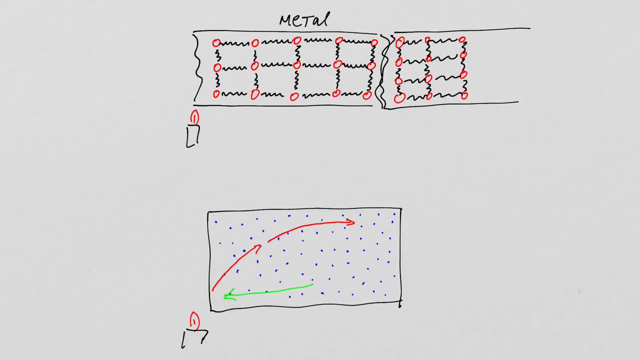 They collide with the hot walls, They get energized, They move away. More cold molecules come this way, They get energized and move this way, And so essentially what you get is a current of molecules that circulates like this And that circulates like so. 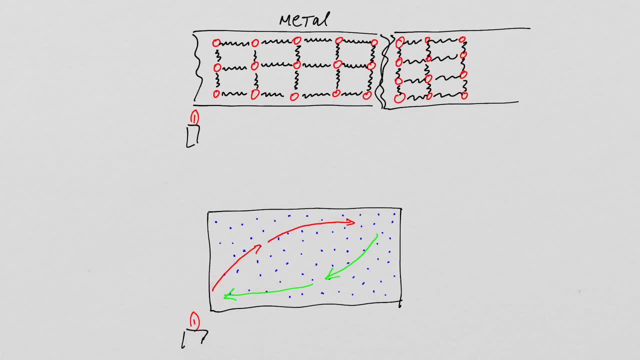 And this current is known as convection current And on a large scale, wind is essentially convection current. It happens when there is difference in temperatures in two regions of the atmosphere, which causes the air molecules to sort of circulate like this: 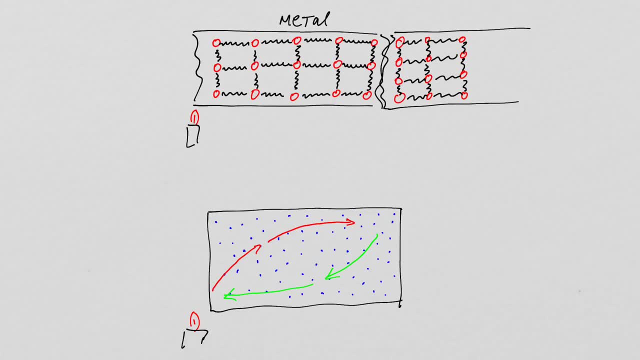 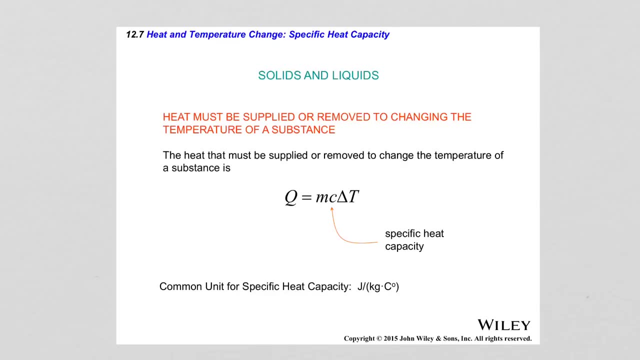 So this is the mechanism of heat transfer inside fluids, so gases and liquids. In order to change the temperature of a substance, solid or liquid substance, heat must be supplied or removed for this change to occur. So consider, you have a substance with the mass M. 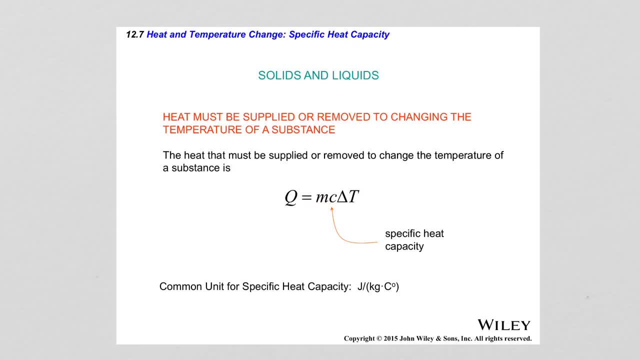 and you are looking to change the temperature of that substance by the amount of delta T. So the amount of heat that is necessary to be supplied or removed for that change in temperature to happen is calculated as the product of the mass of the substance, the specific heat capacity of that substance. 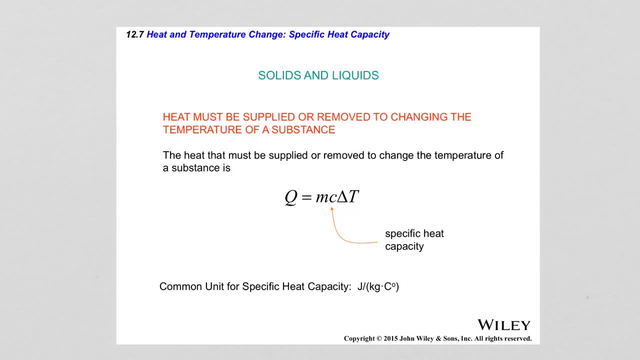 and the change in temperature. A common unit for the specific heat capacity C is joules per kilogram Celsius degrees, And this amount of heat will be either a positive number or a negative number depending on the change in temperature. So, for example, 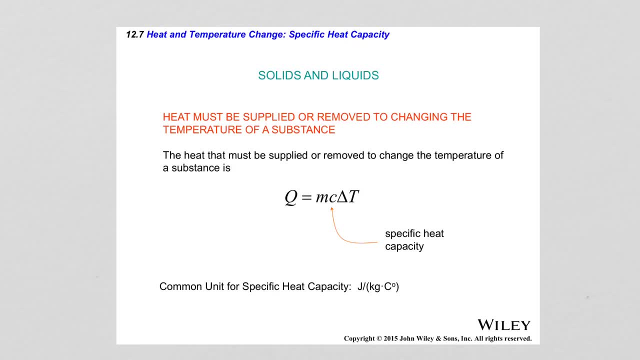 if the substance starts with low temperature and then the temperature is increased, this change in temperature here is positive and therefore the amount of heat will be positive. What does that mean? It means that in order to change the temperature of the substance from lower to higher, 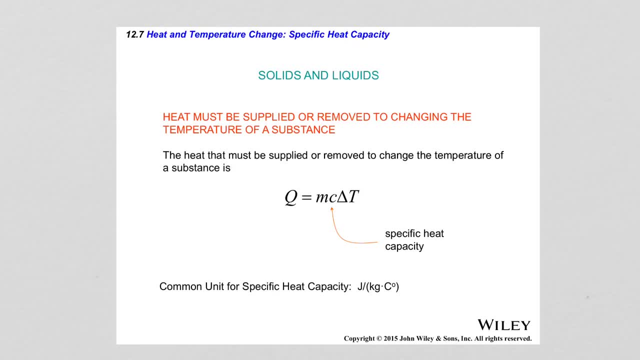 heat must be added to the substance, So that's why a positive quantity. However, if the change in temperature is negative, meaning the initial temperature is higher than the final temperature, then this amount of heat will be a negative number. What does that mean physically? 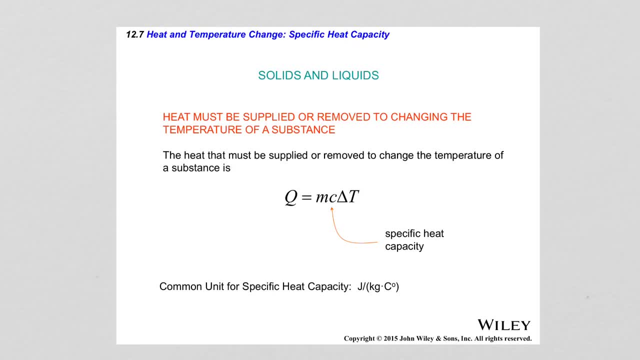 It means that in order for the temperature to decrease, heat must be removed from the substance. So that means negative change in temperature and that is a negative amount of heat. So when heat is added to a substance to increase its temperature, that amount is positive. 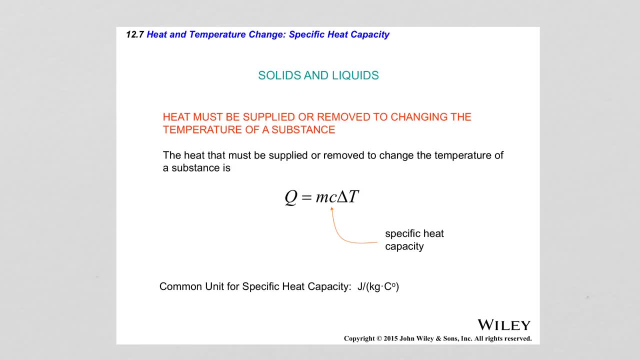 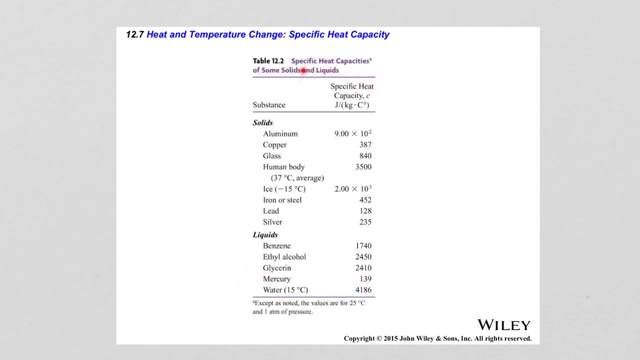 When heat is removed, that amount is negative. So it's important to keep track of the signs of the amounts of heat added or removed in order to get your results correct when you do calculations. In this table, the specific heat capacity is presented for various substances. 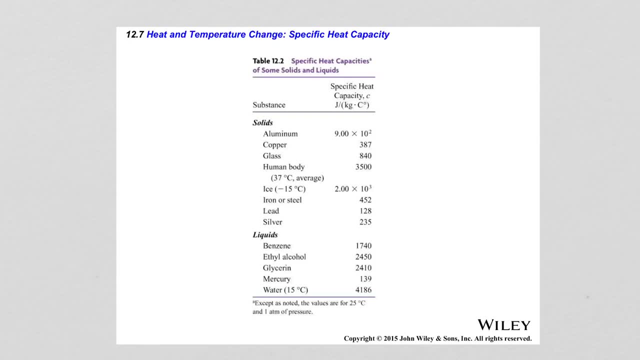 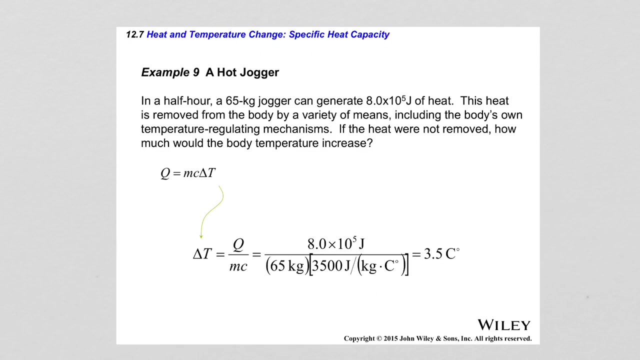 And, as you can see, each substance has its own specific heat capacity, And so the specific heat capacity is actually a good identifier for various substances. No two substances have the same specific heat capacity. Let's look at the following example illustrating the application of the definition of heat. 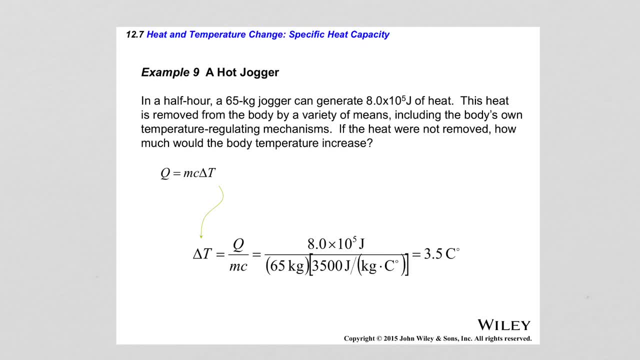 In a half hour, a 65 kilogram jogger can generate 8 times 10 to the fifth joules of heat. This heat is removed from the body by a variety of means, including the body's own temperature-regulating mechanisms. If the heat were not removed, 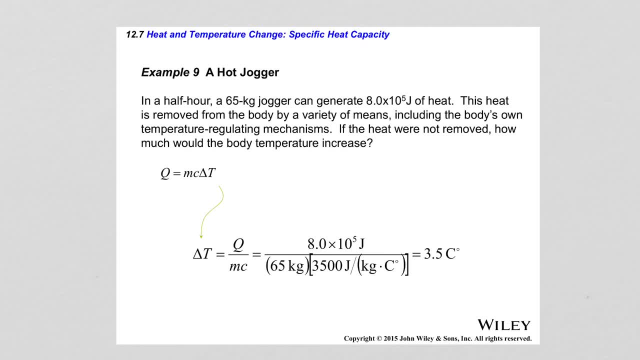 how much would the body temperature increase? So we know that the amount of heat necessary for a specific change in temperature is calculated as the product of the mass of the substance times the specific heat capacity times the change in temperature From the table on the previous page. 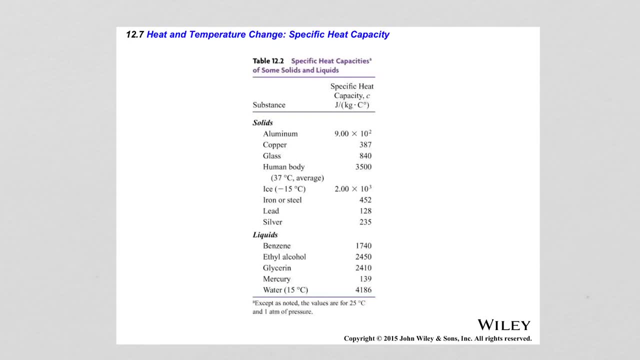 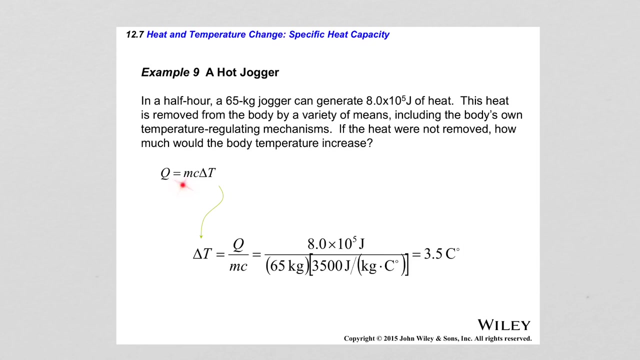 we see that for the average human body at standard body temperature of 37 degrees Celsius, the specific heat capacity is 3500 joules per kilogram degrees Celsius. So rearranging the terms in the formula to solve for the change in temperature gives me Q divided by M times C. 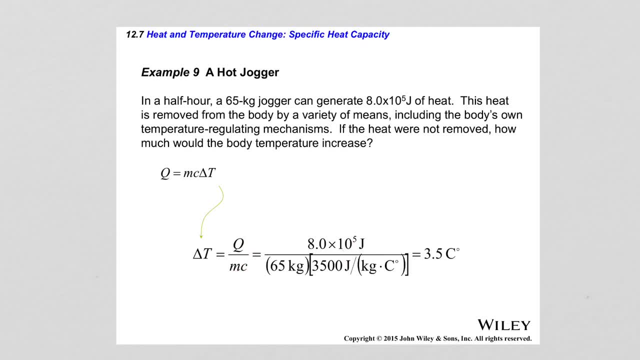 So that is 8 times 10 to the fifth joules divided by 65 kilograms times 3500 joules per kilogram degrees Celsius, which gives me that the change in temperature will be 3.5 Celsius degrees. So if this jogger didn't lose any heat, 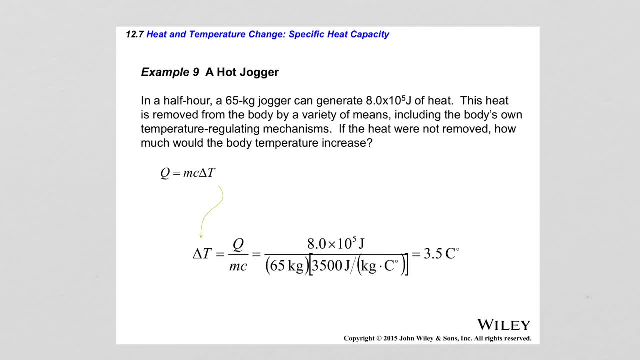 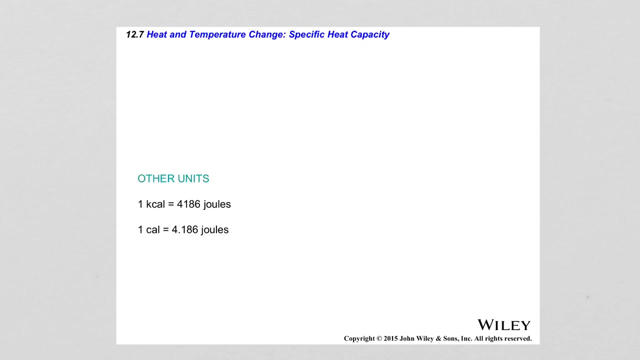 while running they would feel as if they had fever, because 37 plus 3.5, that is 40.5 degrees Celsius. That is equal to 102.9 degrees Fahrenheit. That's as if you're having fever, Since heat is defined as energy flow. 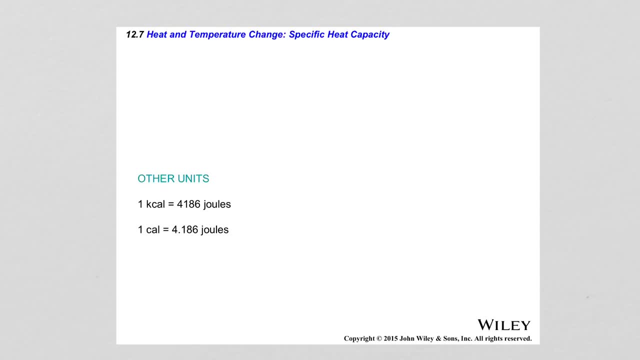 between hotter and colder objects. heat is measured in joules. However, there is another unit that is used historically for heat, and that is the calorie, And one calorie is defined as the amount of heat necessary to heat up one gram of water by one degree Celsius. 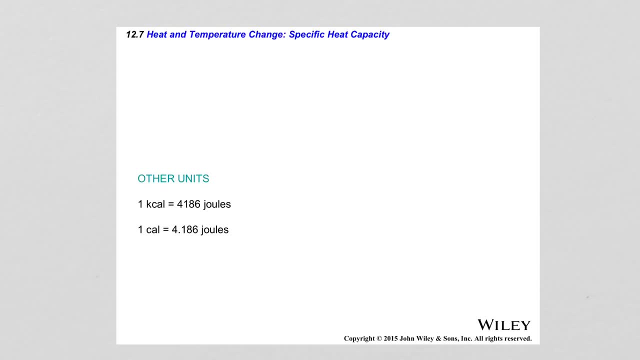 Another unit that is also used is the kilocalorie, which is equal to 1000 calories, and this is the amount of heat necessary to heat up one kilogram of water by one degree Celsius. So what is the relationship between calories and joules? 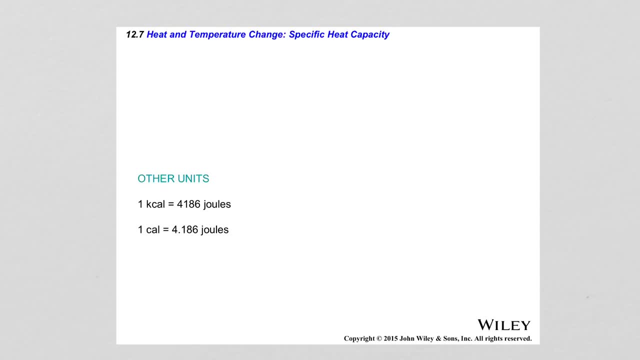 or kilocalories and joules. This relationship was discovered by James Joule- hence the unit joules that are used for energy and work- And what he did was the following experiment: James Joule took a vessel and filled it with water. 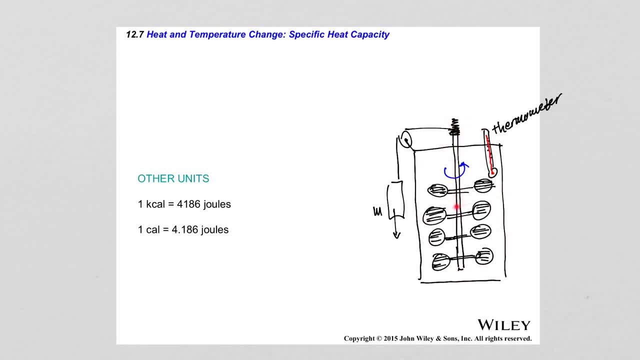 and then inserted a post or a shaft equipped with some paddles and then he connected the free end of the shaft with a hanging mass and when the mass would fall down towards ground, that would cause this shaft here to rotate. that would agitate the water. 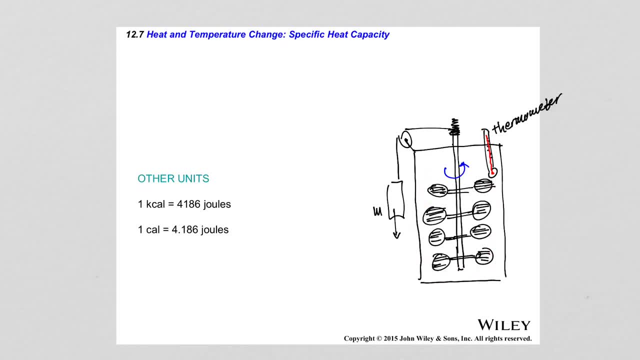 inside the vessel. Well, what James Joule found was that the temperature of the water increased as the mass fell to the ground. That meant that there was some sort of relationship between the work done by the gravitational force on this mass and the heat energy. 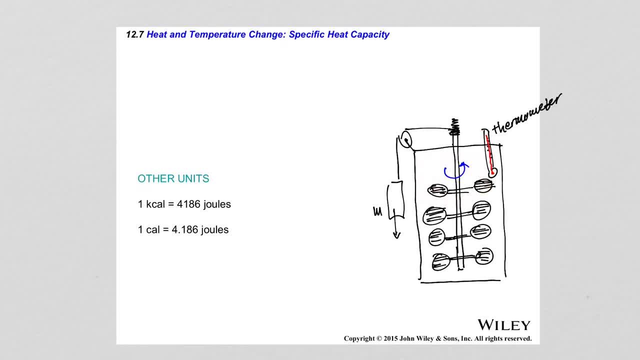 that was transferred to the water, And this relationship is known as mechanical equivalent of heat. The mechanical equivalent of heat states that one calorie of heat is equal to 4.186 joules of work and one kilocalorie of heat is equal to 4,186 joules. 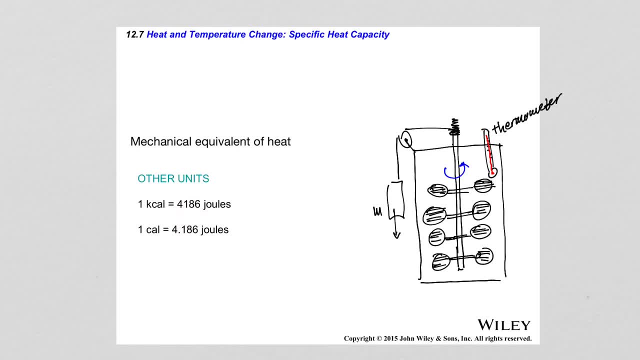 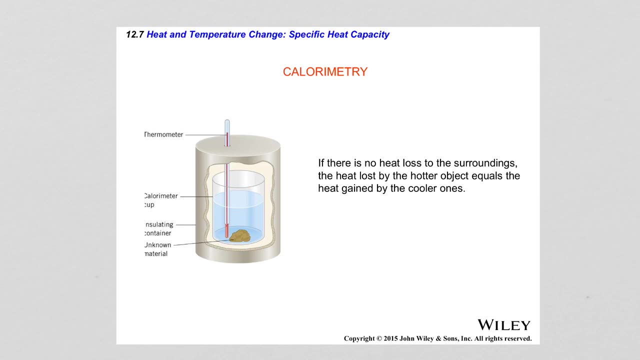 This relationship is important to remember and you must add this to your formula sheets for reference when you do tests. When heat is transferred between a hot and a cold object, it is possible to measure the exact amount of heat transferred if there is no contact with the surroundings. 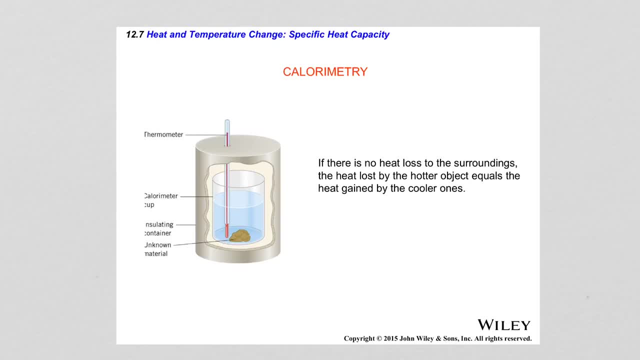 of the system of two objects. The subject of thermophysics that deals with those measurements is called calorimetry. So here is an example of a simple device known as a calorimeter, which is used to measure the amount of heat transferred between a hot and a cold object. 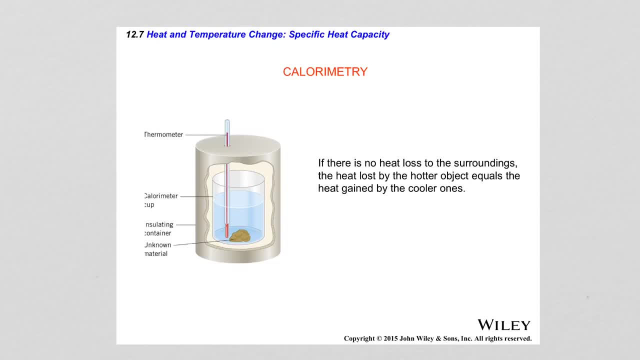 So we have a piece of unknown material that is submerged in a vessel filled with some water, And if this material contains a certain amount of heat, it is at a higher temperature than the water in the vessel When this material is submerged in this vessel. 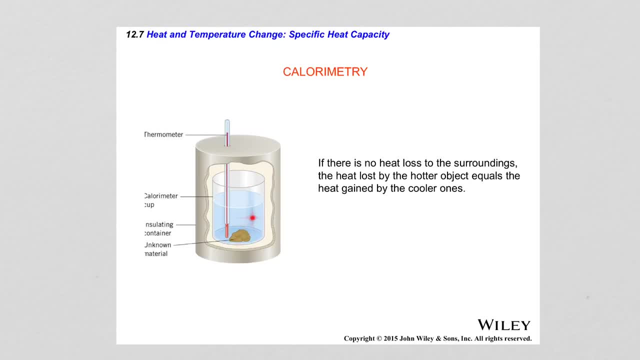 some of the heat energy is going to be transferred to the water, and then the temperature of that water can be measured, And then a calculation can be performed to identify how much heat was transferred from this material to the water. So for this measurement to be successful, 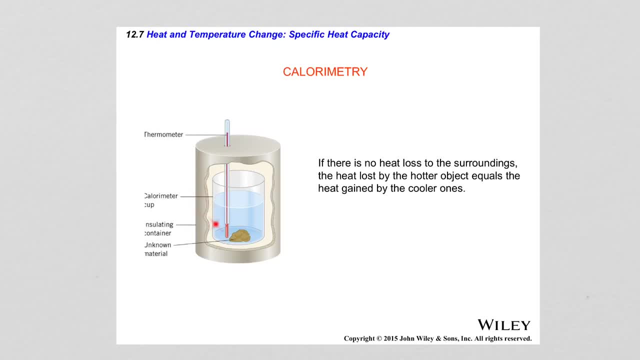 the requirement is that the system, which is the water, the glass vessel, the thermometer and this unknown material, that system must be isolated from the surroundings, So the calorimeter has an insulating wall that prevents heat exchange with the outside of the system. 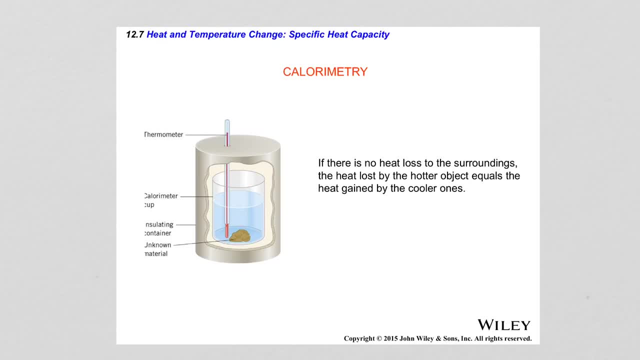 And so, based on the measurements of the initial temperature of the water and the material, the final temperature of the water and the material and the properties of water and glass, one could calculate how much heat was released by by this unknown material to the water. 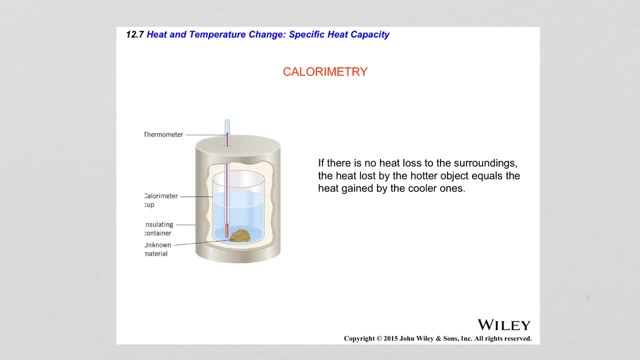 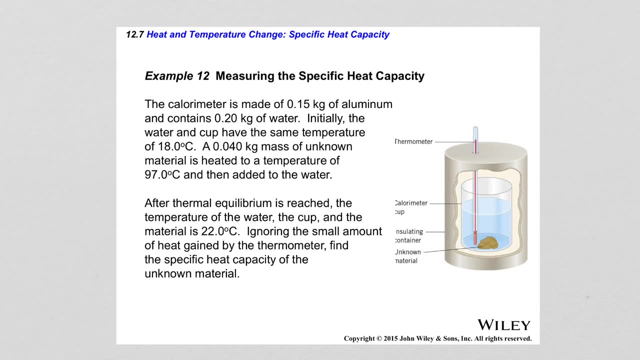 From that calculation one could also calculate what type of material that is, or identify what type of material that is by calculating the specific heat capacity of that material. Here is an example that shows how a calorimeter works: The calorimeter shown here in the drawing. 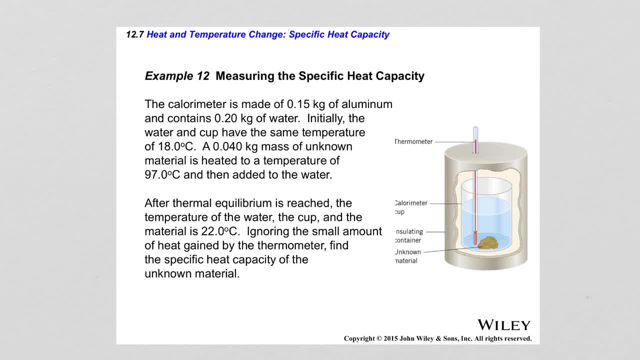 is made of 0.15 kilograms of aluminum and contains 0.2 kilograms of water. Initially the water cup have the water and the cup have the same temperature of 18 degrees Celsius. A 0.04 kilogram mass of unknown material. 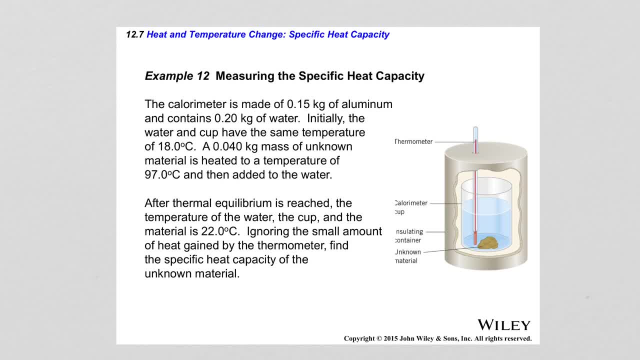 is heated to a temperature of 97 degrees Celsius and then added to the water After a thermal equilibrium is reached. the temperature of the water, the cup and the material is 22 degrees Celsius, Ignoring the small amount of heat gained by the thermometer. 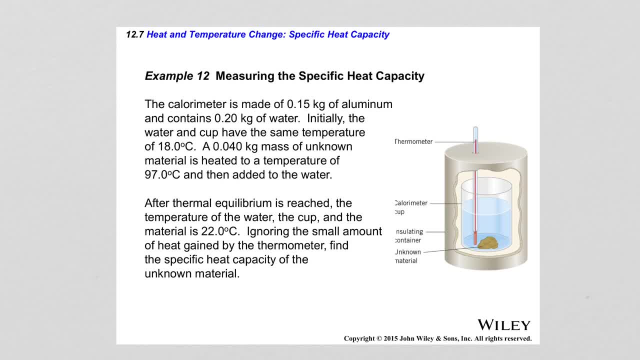 finds the specific heat capacity of the unknown material. So the heat that is contained, the heat energy that the unknown material is going to release into the calorimeter, is going to go towards heating up the calorimeter and heating up the water in the calorimeter. 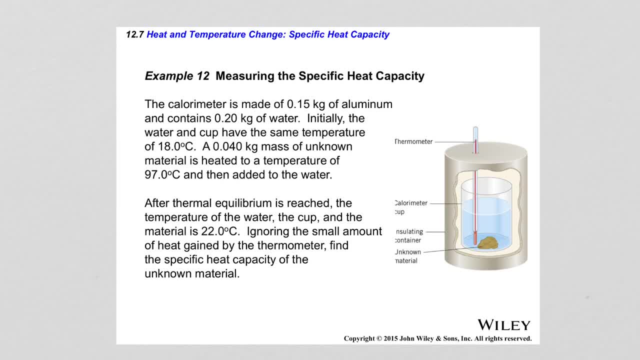 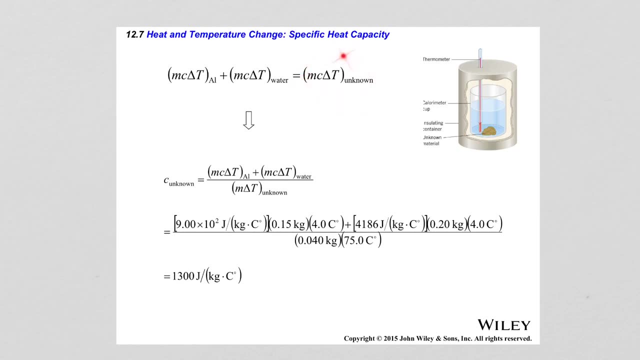 When all of these three members of the system have the same temperature, then thermal equilibrium is reached and no longer heat exchange is happening. So that means that the amount of heat that the unknown material is going to lose will be equal to the amount of heat. 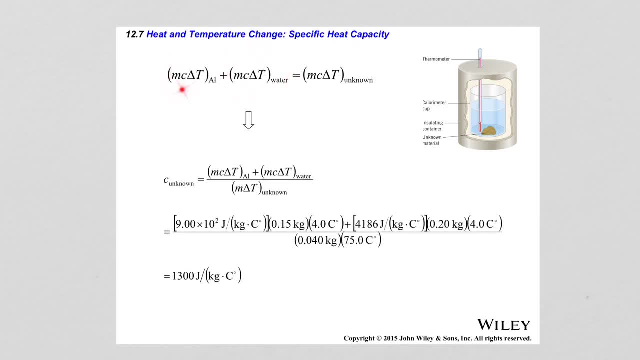 that the water in the calorimeter will receive, plus the amount of heat that the aluminum, the material from which the calorimeter is made, will receive. So from this I can solve for the specific heat of the unknown material which gives me this relationship. 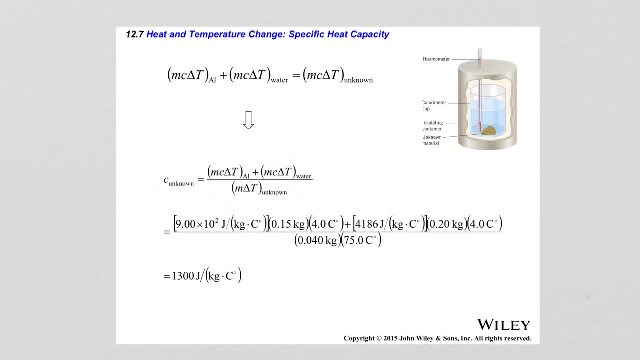 Now I know the masses of the water, of the aluminum and the water, I know the specific heats of aluminum and water and I know the change in temperature of aluminum and water. I also, of course, know the mass of the unknown material. 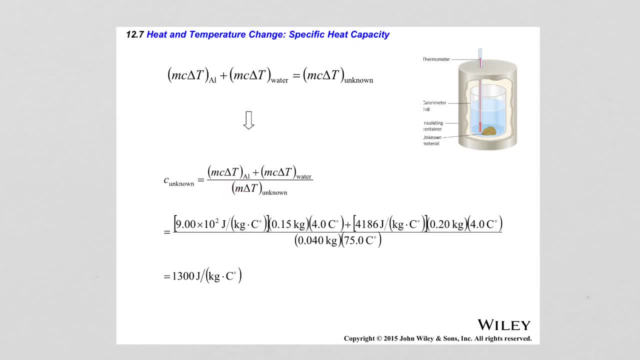 and I know the change in temperature of the unknown material. So when I plug in all these numbers here, the result is that the specific heat of the unknown material is 1300 joules per kilogram Celsius degree. So that corresponds to: 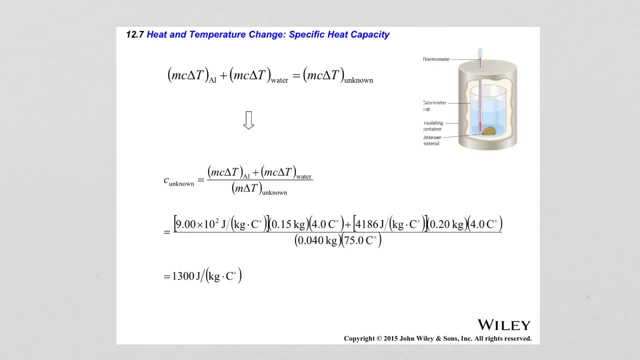 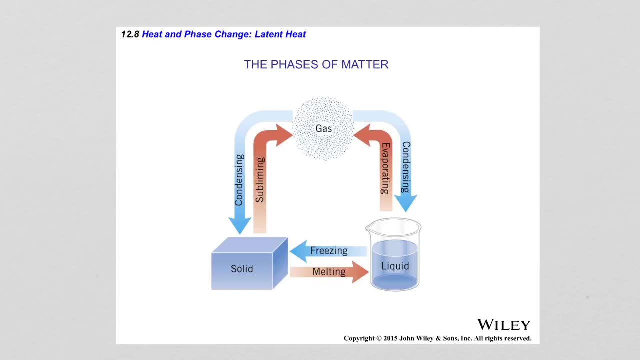 that corresponds to wood pulp type of material. There are situations in which the addition or removal of heat does not cause temperature change. Those situations are situations where a certain substance changes phase, which means it transitions from a solid into liquid state or from liquid state to gaseous state. 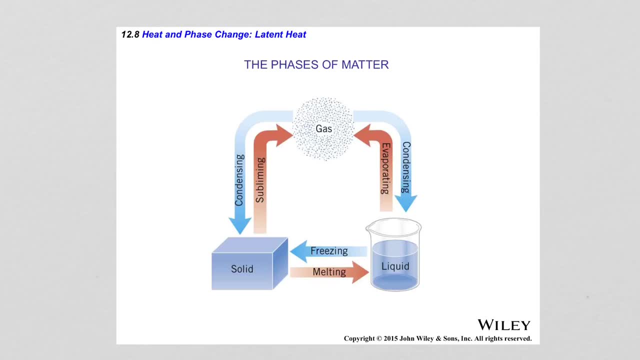 or the other way around, from gaseous to liquid state, from liquid state to solid state, or from gaseous straight to solid, so on and so forth. So these types of transitions are called phase changes, And so during a phase change, 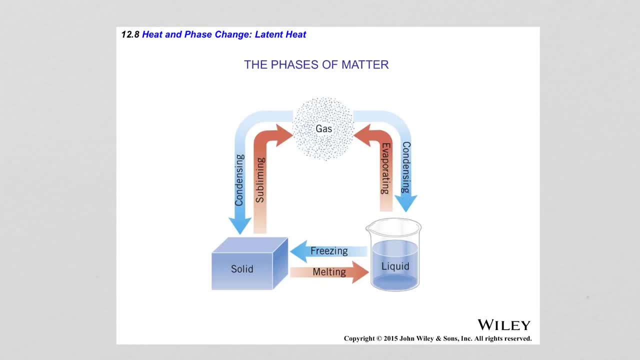 the temperature of the substance remains constant even though heat is being exchanged for the change to happen. Here in this drawing are shown all the possible changes of phase between various states of matter. So solid can sublimate into gas and then gas can condense back into solid. 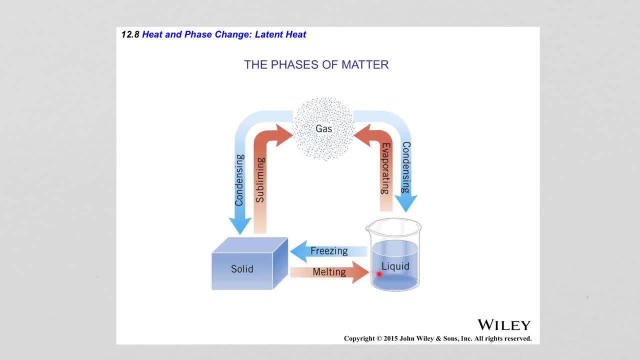 So this is a reversible process. Solid can melt into liquid. liquid can be frozen into solid. also a reversible process: Liquid can evaporate into gas and gas can condense into liquid. Reversible process For all of these processes in either direction. 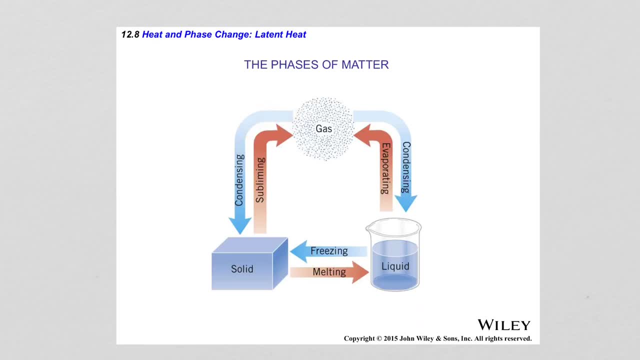 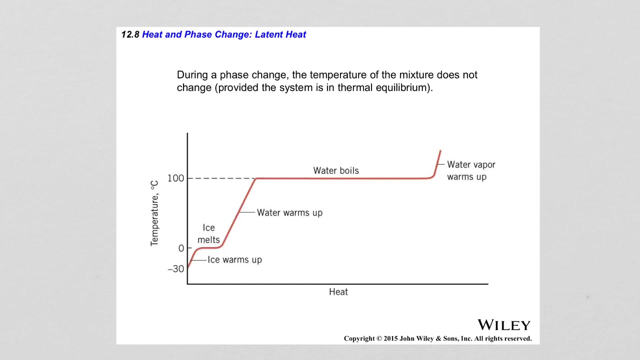 the same amount of heat is exchanged, either added or removed, depending on which direction the phase change is happening. However, during those transitions, the temperature of the mixture remains constant. So here is a plot of temperature versus heat for the transitions of water. 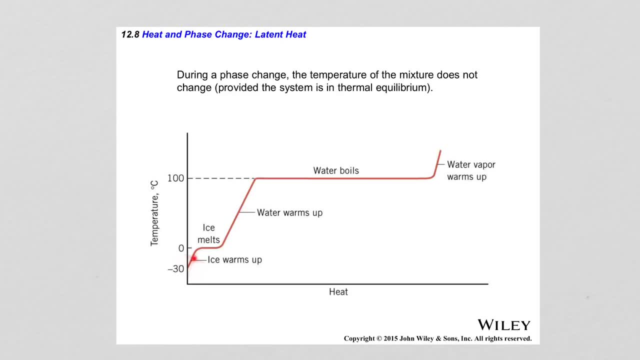 So if we start with ice, ice is obviously a solid. when it reaches zero degrees Celsius, it starts to melt. During that melting process, ice remains at zero degrees temperature Only after all of the ice has melted. the temperature of the water now starts to rise. 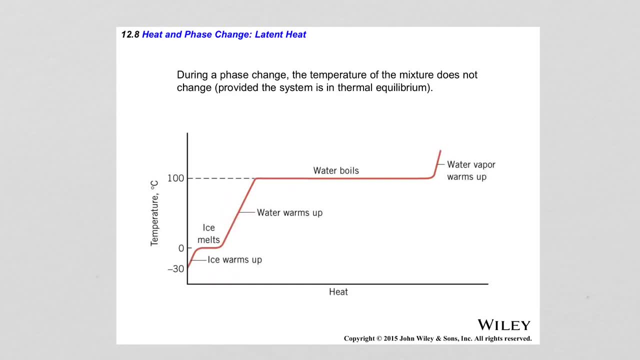 So, as heat is being added, temperature starts to rise until it reaches a boiling point. At that moment, no matter how much heat is being added to the boiling water, the temperature of the boiling water will remain the same. It will be at 100 degrees Celsius. 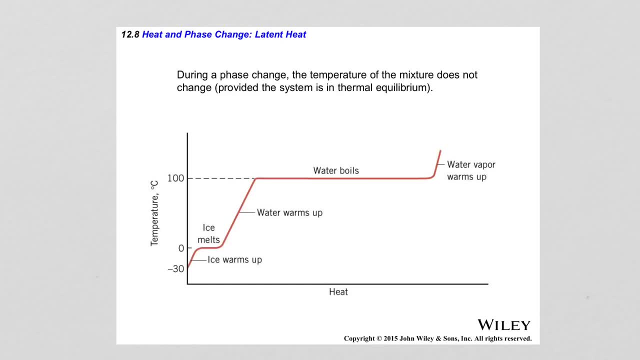 Only after all of the water has boiled and turned into steam or water vapor will the temperature of that steam or water vapor start to increase again. So during those transition periods here or sections where we have phase change, we have a mixture at the same time. 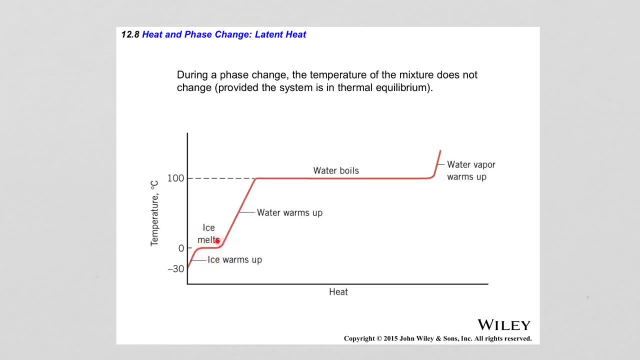 of- here ice and water and here boiling water and steam. The mixture is at the temperature of transition, which is zero degrees Celsius for ice-water mixture and 100 degrees Celsius for water and steam mixture, So the same applies for any other substance. 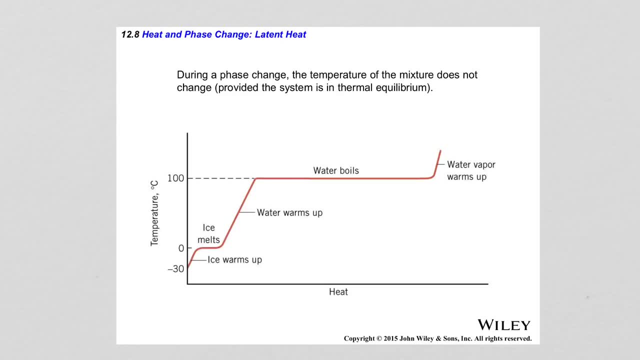 except for these temperatures, of course, will be something else. So the most important takeaway here is that during phase transition, the temperature of the mixture where the two phases coexist is constant. So, for example, if you grab some ice and you put it in water, 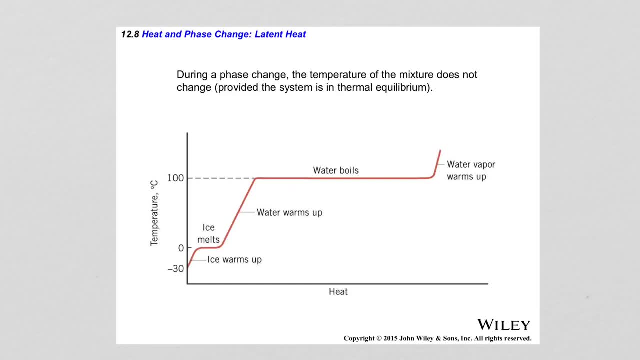 once the temperature equilibrates, you will find out that the ice-water mixture is at zero degrees Celsius. Of course, if you let it be for a while, heat is going to be absorbed from the surroundings. That is going to cause the ice. 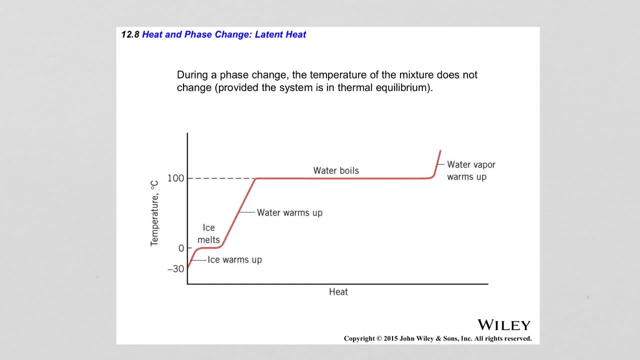 to melt, and once the melting has stopped now, the temperature of the water only will start to increase. The amount of heat that must be supplied or removed to change the phase of a substance is calculated as the product of the mass of that substance times this new quantity. 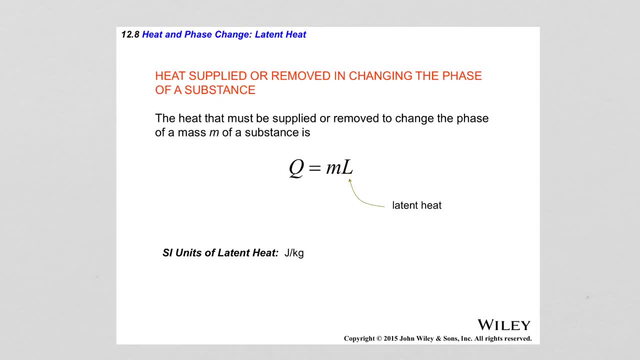 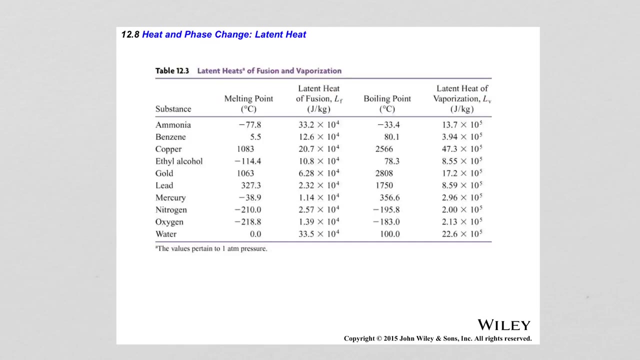 which is called latent heat. This quantity latent heat has different values depending on the type of phase change that this substance is undergoing. Latent heat is measured in units of joules per kilogram, And here is a table with latent heat. 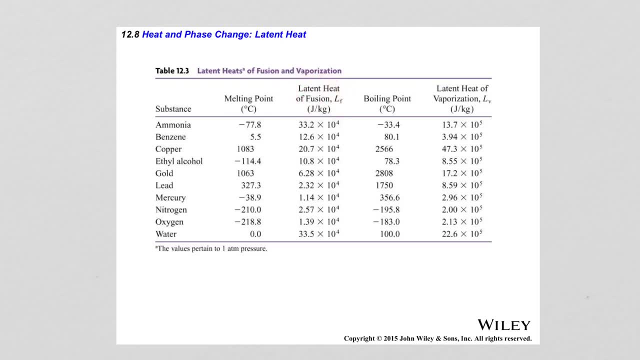 of fusion, which is the latent heat necessary for phase change from liquid to solid or solid to liquid, And also the values for the latent heat of vaporization, which is the latent heat necessary for transitions from liquids to vapors or the other way. 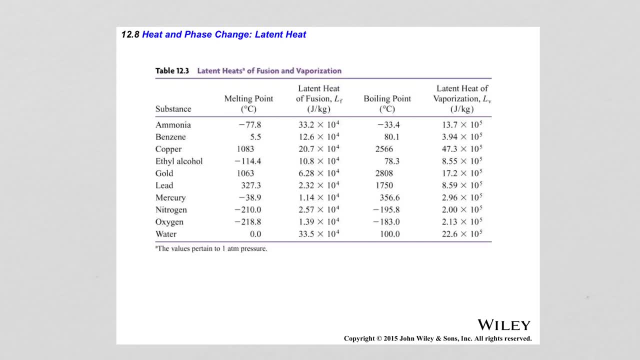 from vapors to liquids or gases to liquids. So, depending on the phase transition from liquid to solid or solid to liquid- we talk about latent heat of fusion. And if we have transition from liquid to gas or from gas to liquid, 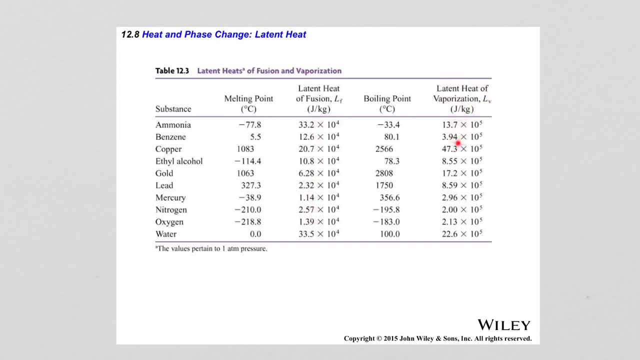 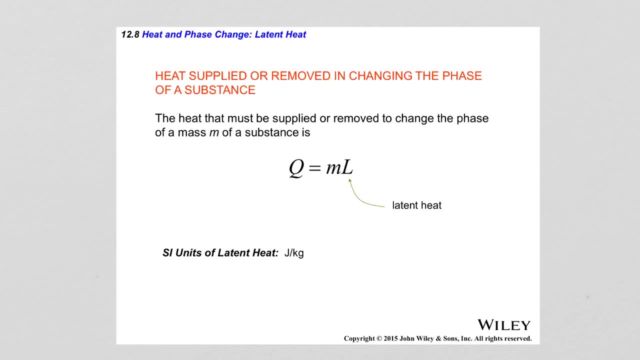 we talk about latent heat, of vaporization, And so these are the values for those two types of latent heat for several different substances. So if you are calculating how much heat was necessary to melt a certain amount of, let's say, copper, for the latent heat here, 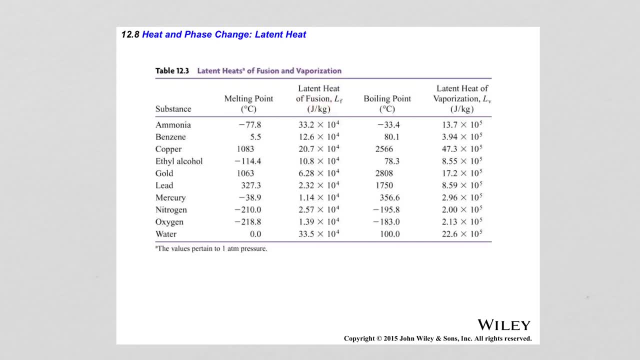 you would use latent heat of fusion, and for copper that is 20.7 x 10⁴. Now if you were evaporating, let's say, benzene, then the amount of heat necessary to evaporate a certain amount of benzene 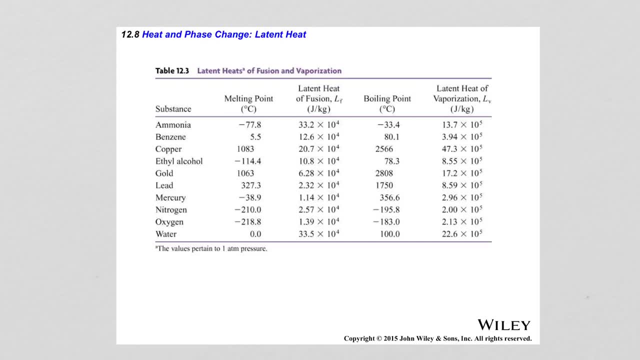 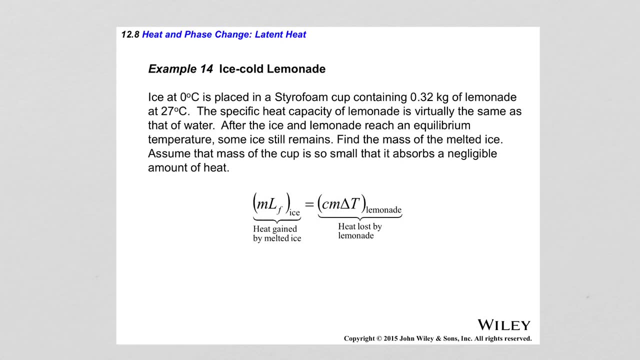 would be calculated by using the latent heat of vaporization, which is 3.94 x 10⁵. Here is an example that illustrates the concept of latent heat: Ice at 0°C is placed in a styrofoam cup containing 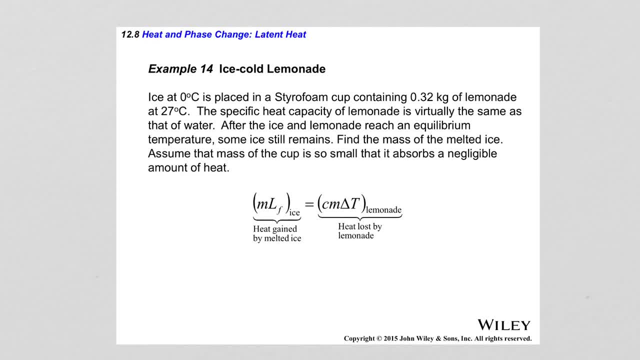 0.32 kg of lemonade. at 27°C, The specific heat capacity of lemonade is virtually the same as that of water. After the ice and lemonade reach an equilibrium temperature, some ice still remains. Find the mass of the melted ice. 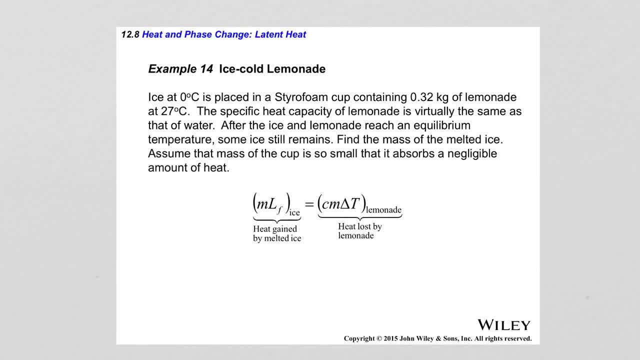 Assume that the mass of the cup is so small that it absorbs a negligible amount of heat. So this equation, this problem is about conservation of energy. The amount of heat gained by the melting ice must be equal to the amount of heat lost by the lemonade. 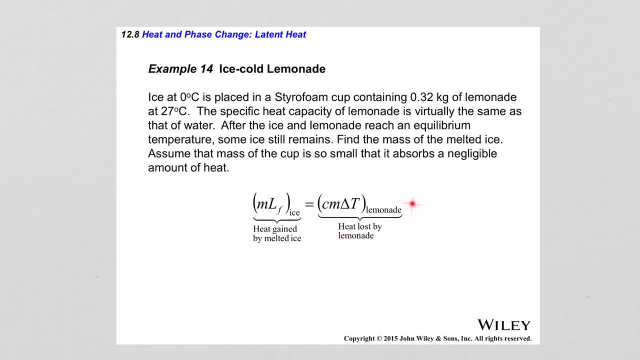 The amount of heat lost by the lemonade is calculated by the formula that we discussed a few slides ago. So that is specific heat of lemonade times the mass of lemonade times the change in temperature due to the heat loss For the melting ice we use. 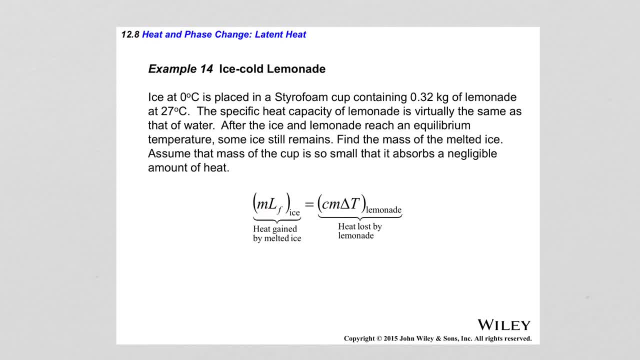 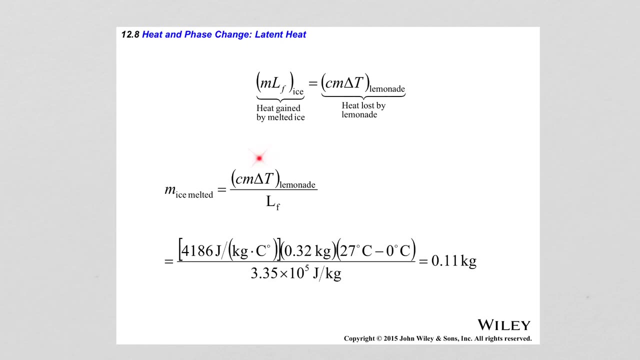 the product of the mass of the melted ice times the latent heat fusion for ice. So those two quantities must be equal. So from here I solve for the melted ice, and that is equal to the amount of heat lost by the lemonade divided by the. 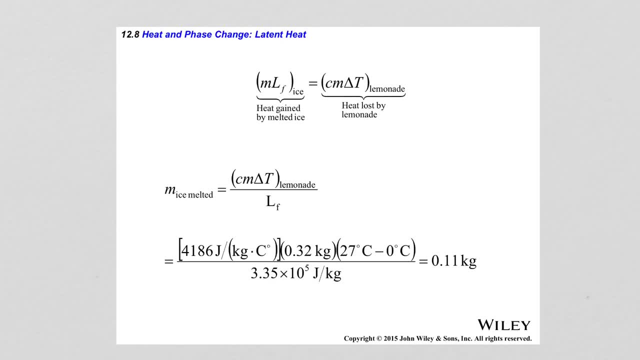 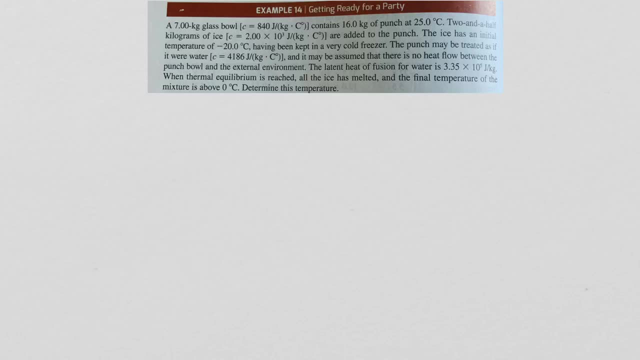 latent heat fusion for ice, That gives me 0.011 kg. Let's do one more example that has a little bit more going on for it To again illustrate the concept of latent heat: A 7 kg glass bowl with specific heat of. 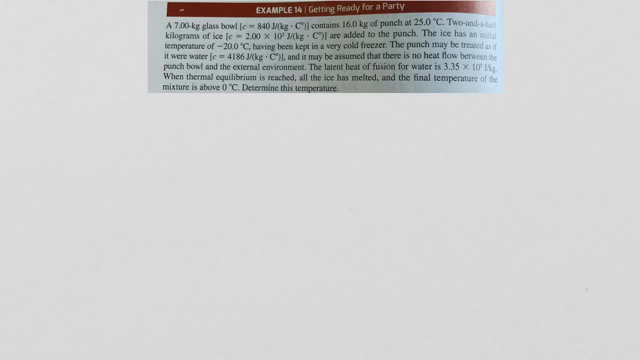 840 Joules per kg C contains 16 kg of punch at 25 C, 2.5 kg of ice with specific heat of 2 x 10 to the 3 Joules per kg C are added to the punch, The ice has an. 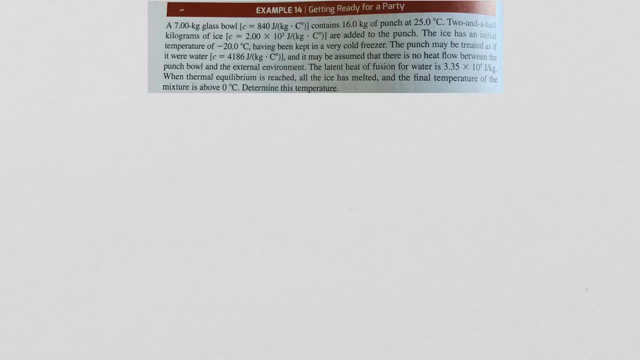 initial temperature of negative 20 C. It is kept in a very cold freezer. The punch may be treated as if it were water with specific heat of 4.186 Joules per kg C, And it may be assumed that there is no heat flow between. 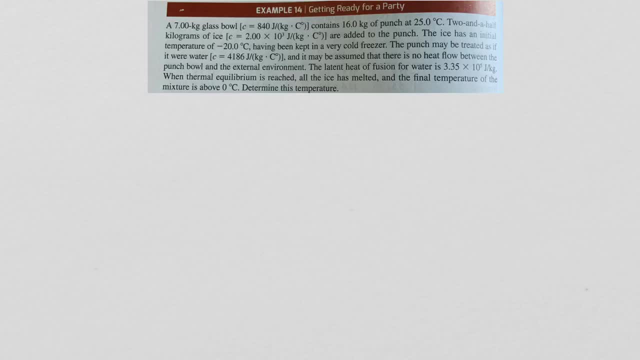 the punch bowl and the external environment. The latent heat of fusion of water is 3.35 x 10 to the 5 Joules per kg C. When thermal equilibrium is reached, all the ice has melted and the final temperature of the mixture is above 0 C. 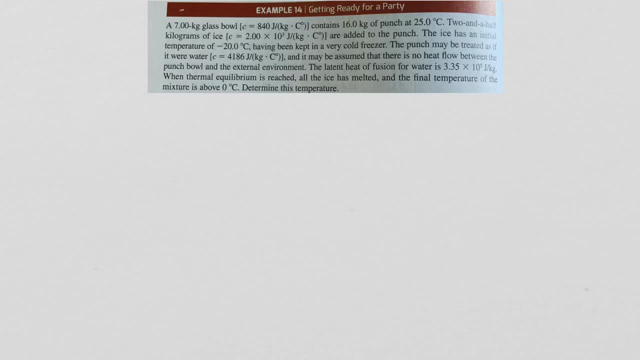 Determine this temperature. So this is a problem again about conservation of energy. The amount of heat that was lost is equal to the amount of heat that was gained. So let's see what the gained heat is. Where does it go? So the gained heat? 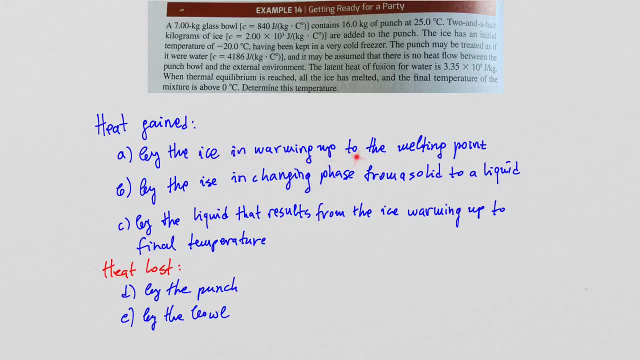 is first by the ice in warming up the melting point, Second by the ice in changing phase from a solid to a liquid And lastly by the liquid that results from the ice warming up to its final temperature. The heat is lost by the punch and also by 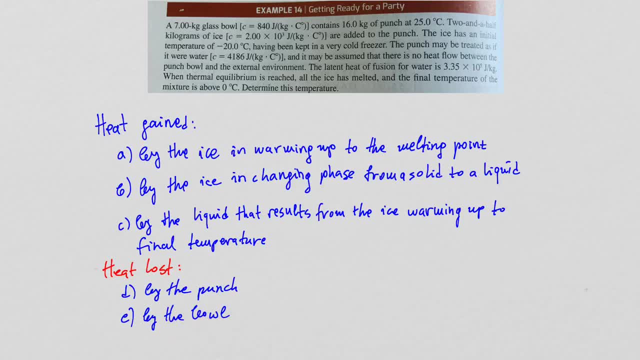 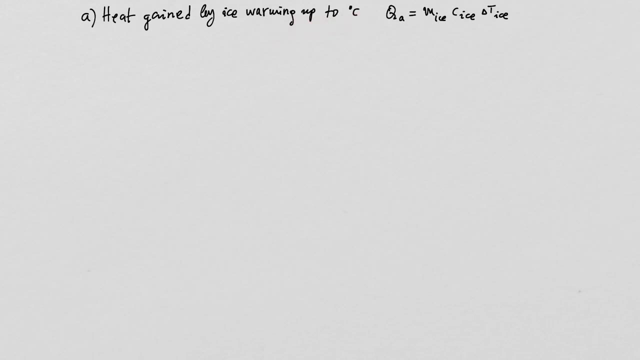 the ball, and both are cooling down as they are losing heat. Now let's calculate the amounts of heat corresponding to each of those situations. So the heat gained by the ice warming up to 0 C is calculated as the product of the mass of the ice times. specific heat applies. 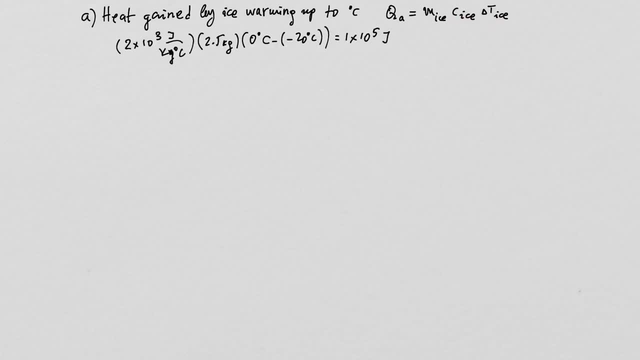 times the change in temperature. So, substituting the values provided in the problem, that gives us 2 x 10 to the 3rd Joules per kg C, times 2.5 kg, times 0 minus minus 20 C, that is equal to: 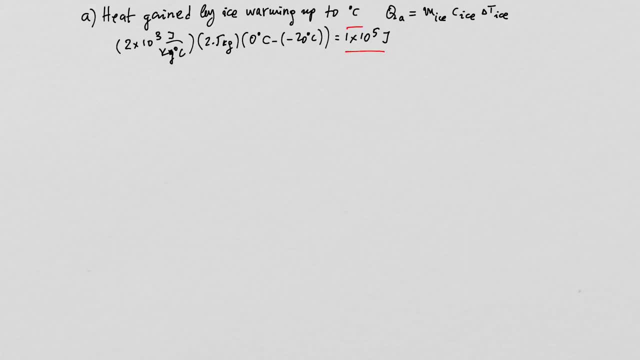 1 x 10 to the 5th Joules. Now let's calculate the next one, which is the heat gained when the ice melts at 0 C. So this is a phase transition. So the heat that is gained by the ice when it melts at 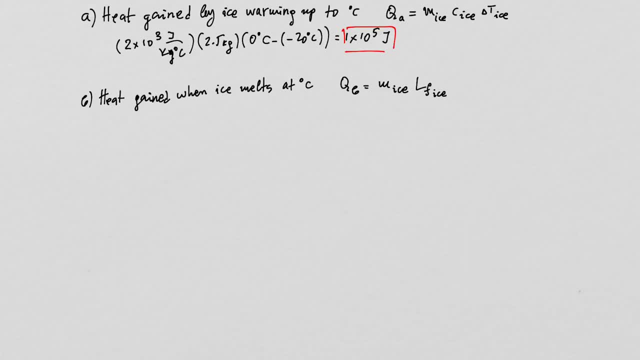 0 C, 0 C. 0 C is calculated as the product of the mass of ice times the latent heat diffusion for ice. So that gives us 2.5 kg x 3.35 x 10 to the fifth Joules per kg. 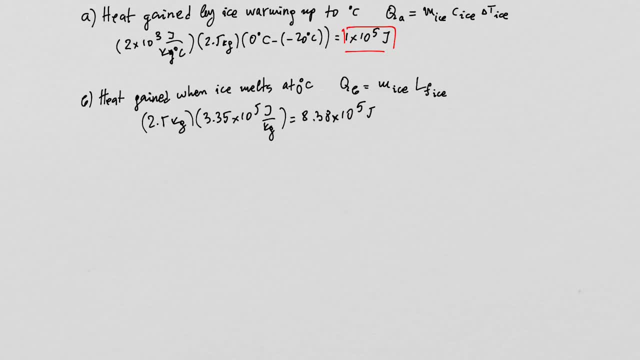 8.38 x 10 to the fifth Joules. Next, let's calculate the heat gained when the melted ice, which is now liquid, warms up to a final temperature of T, which is what we are looking for. that final temperature T of heat Qc is equal to the mass of ice times the specific heat of water. 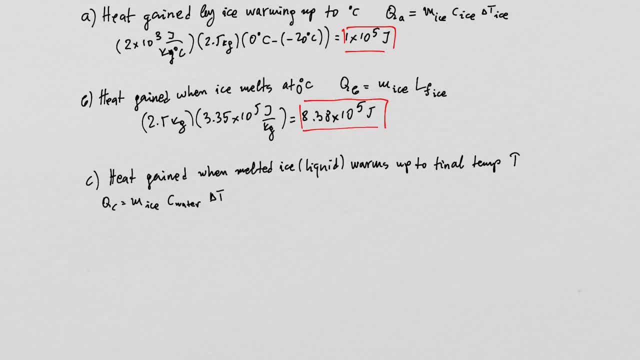 remember, the ice has melted so it's liquid now, meaning water times the change in temperature. So that amount of heat is equal to 2.5 kilograms times 4,186 joules per kilogram degrees Celsius. that's the specific heat of 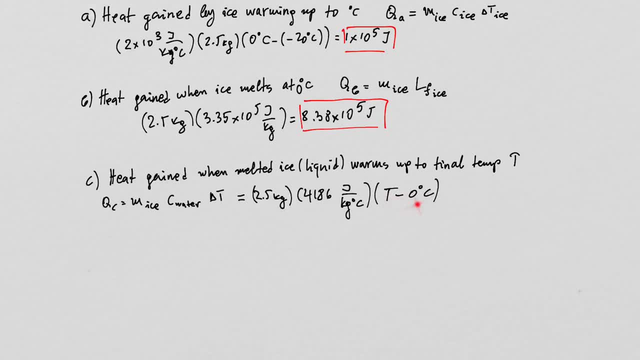 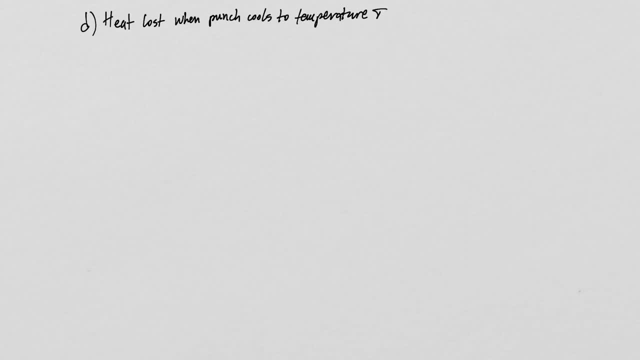 water times T minus zero degrees Celsius. that's the temperature difference. I'm done with the heat gained portion of the calculation. now let's look at the heat lost portion of the calculation. So first we have the heat lost when the punch cools down to a temperature T, So that is calculated as the mass of punch. 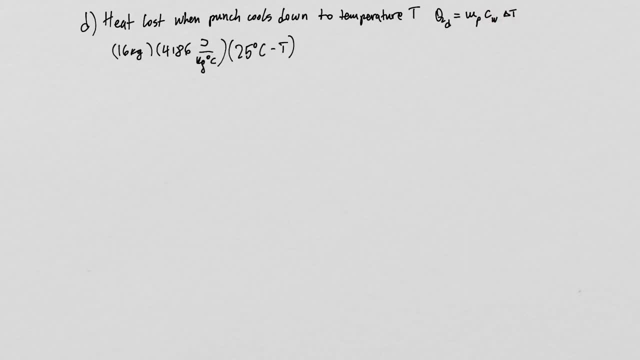 times the specific heat of water, times the change in temperature. So that gives me 16 kilograms times 4,186 joules per kilogram degrees Celsius, times 25 degrees Celsius minus T. And finally I need to also calculate the heat lost by the. 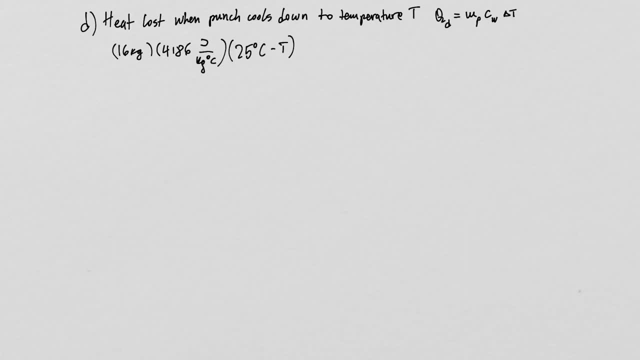 ball when it cools to temperature T, So that heat is equal to the mass of the ball times the specific heat of the ball times the change in temperature. This gives me 7 kilograms times 840 joules per kilogram degrees Celsius times 25. 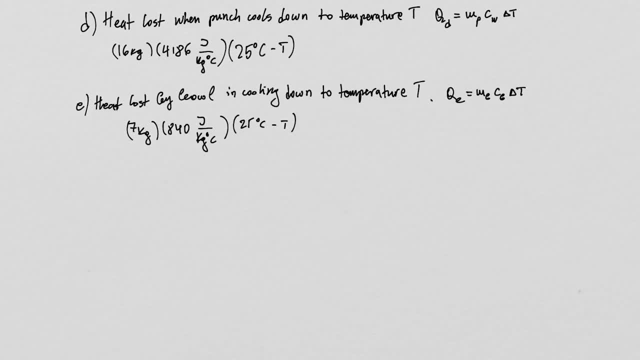 degrees Celsius minus T. The ball and the punch both start at the same temperature- 25 degrees Celsius- and both end at the same temperature, T. So now, conservation of energy requires that all the amounts of heat gained- the calculated amounts of heat in points A, B and C added together- must be equal to the 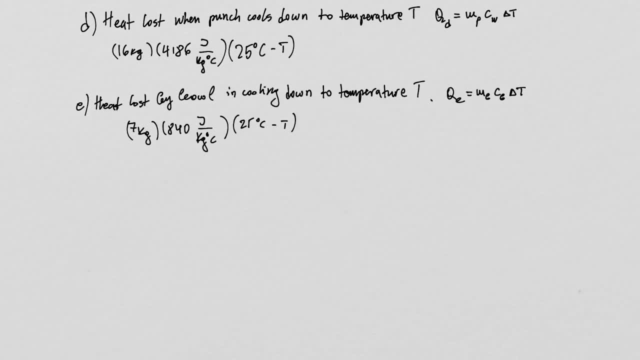 amount of heat lost, calculated in D and E. So again, the amount of heat gained- QA plus QB plus QC- must be equal to the amount of heat lost, which is QD plus QA. So from here I can solve for the final temperature, T, And so I end up with the. 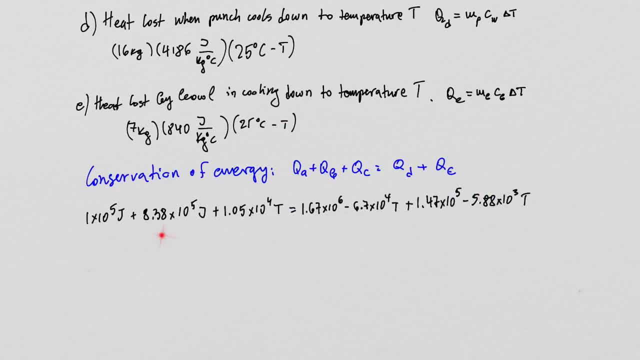 following relationship: The first quantity corresponds to QA, the second quantity corresponds to QB, the third quantity corresponds to QC and then, on the right side, this corresponds to QD and this corresponds to QE. After grouping the terms that have the temperature T in them and doing some simple algebra, the final result of the 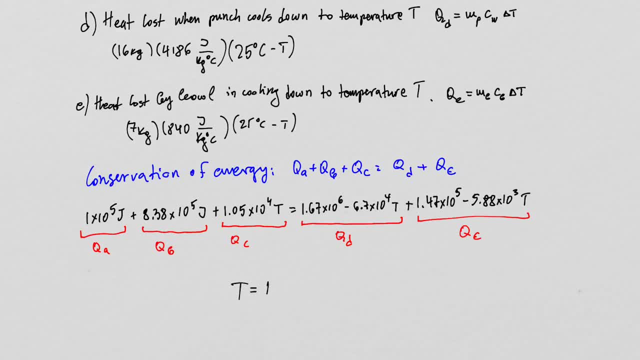 calculation is that the temperature T final is equal to 11 degrees Celsius. So when dealing with those types of problems, it is important to identify the amount of heat gained, the amount of heat lost and what process specifically is happening when heat is being gained or lost, Whether this 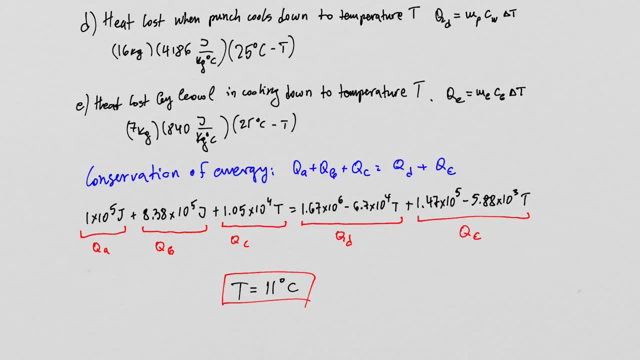 process is just simple heat transfer or just simple heat transfer, or it is a phase change and then apply the definitions for the amount of heat accordingly to get the answer correctly. And so this concludes the lecture on temperature and heat.